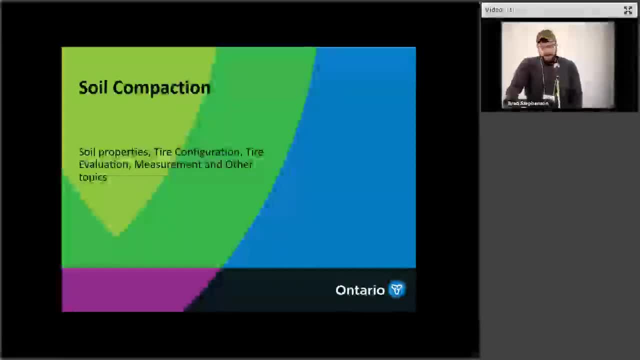 trying to get developed too. So last time I gave this talk, this specific slide deck, it was supposed to be 15 minutes, It took 40 minutes and I didn't get through everything. So who here was at any of the days, either Arthur or- let's see the other one- Elgin or the Dundas? 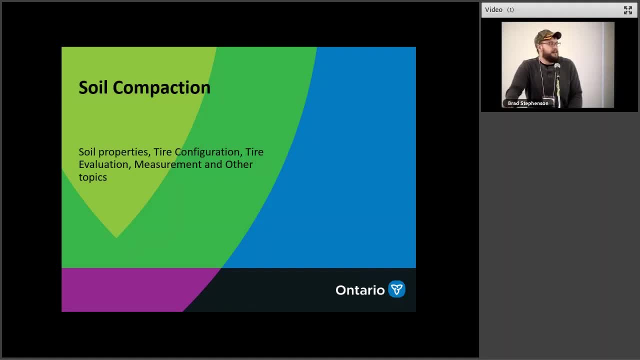 in the east. Alex, If you just put your hand up, do you have any idea what I'm going to be talking about? for the next five minutes? Very few, Okay, Except the one in the middle that's not listening to me, Because I know she was there. 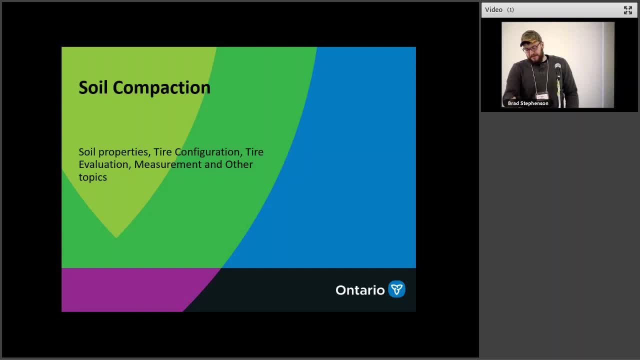 Anyway. so yeah, compaction, soil compaction as a generality. So I'm a mechanical engineer by training and I am a bit of a gear head, So I got to test a bunch of equipment. but now I'm testing a bunch of equipment. 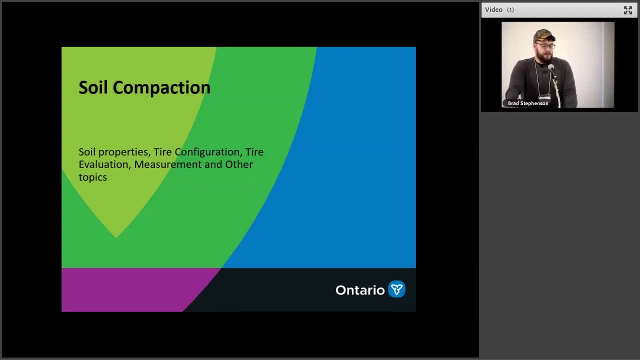 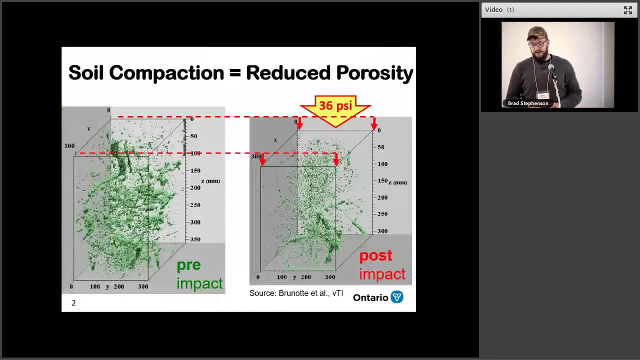 I've got a bunch more equipment but from sort of the standpoint of comparing tires, tracks, high inflation, low inflation or proper inflation anyways, and basically everything we want to know, So the long and short of it is that we don't know very much about it. 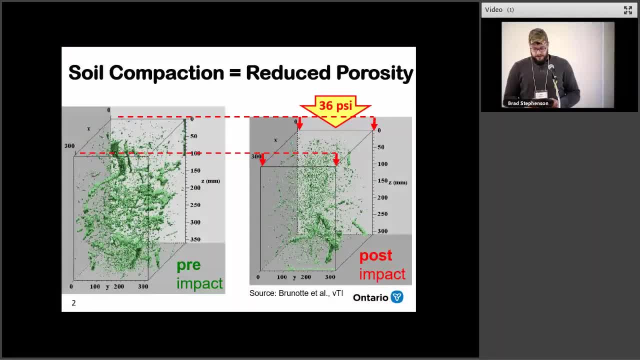 but we do know why it's bad And hopefully we'll get to learn some more about it. So this is a slide from Matthias- well, actually it's from Bruno et al. He presented this, Matthias Stettler presented this and Arthur when we did their when IFAO. 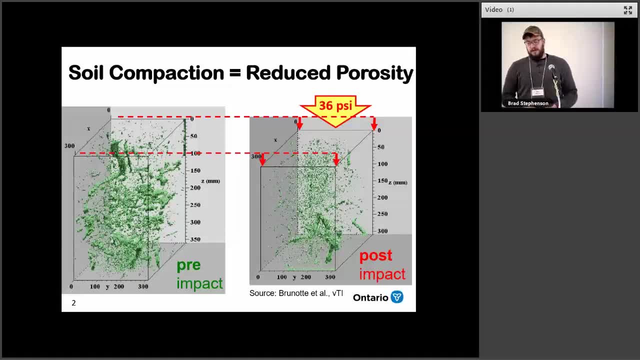 did the first compaction day. So on the left hand side we have a pre-intake soil in a CT scan. So you go to the hospital, you get your CT scan. it tells you where all your bones and stuff are inside. you Do the same with a soil- sample of soil, and you can see all. 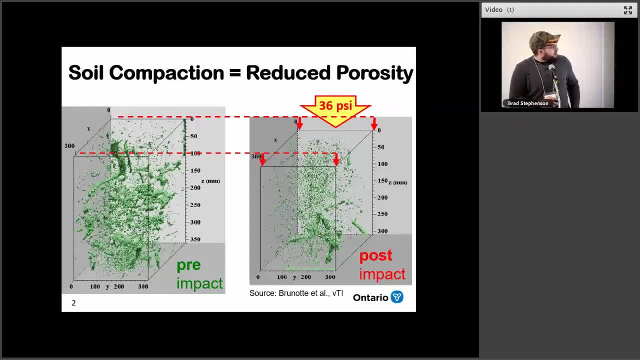 the void space. So all those green lines in there or those green areas are all pore space or open space for air or water to hang out in, and that's kind of what we want. but put a load on it like a tire or anything. in this case it was the. 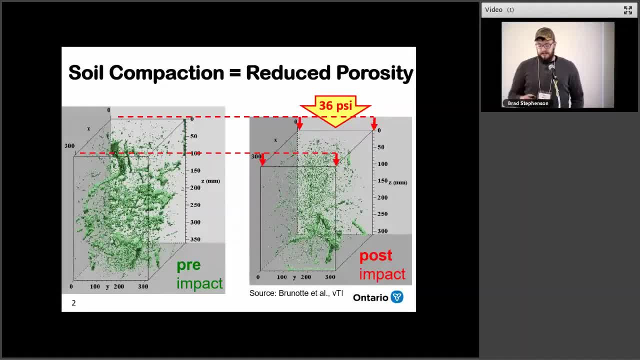 equivalent of 36 psi at the surface of that sample. what do you, what do you see in that second picture- and this is going to be interactive, so make sure you interact with me- the what do you see? there's less, but what else is there? so there's less connectivity. so you see how a lot of that void space went away in. 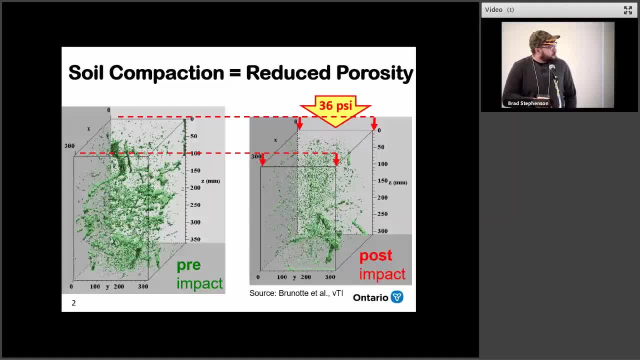 the top half of that sample and not too too much in the in the deep portion of that sample. but there's also less connectivity through the top and the bottom of that sample. so can you imagine trying to get water out of that sample and then you get water out of that sample and then you get? 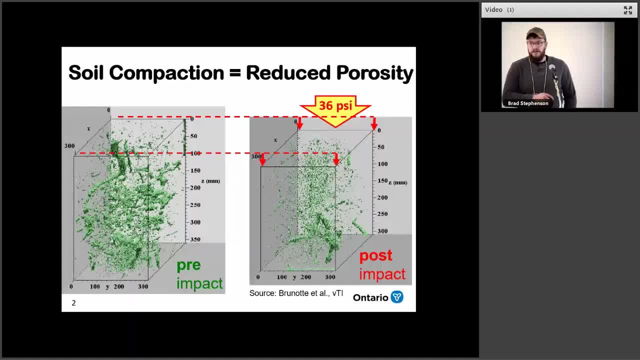 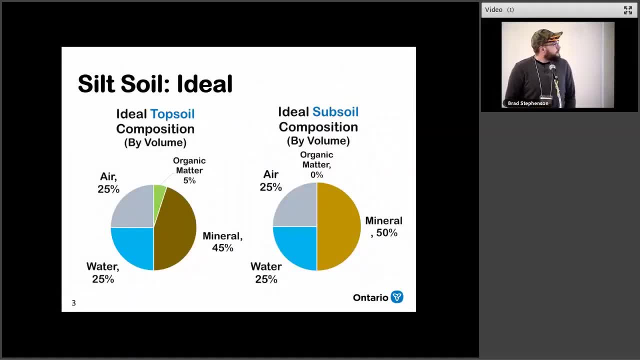 water through this sample or through this sample from top to bottom. there's a lot more connectivity in that first sample on the left. so that's kind of what we're going to talk about for a little while for a silt soil, and just speaking in generalities, which I love doing, because then you don't have to. 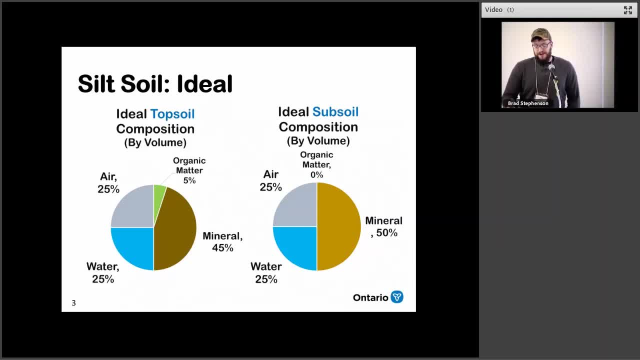 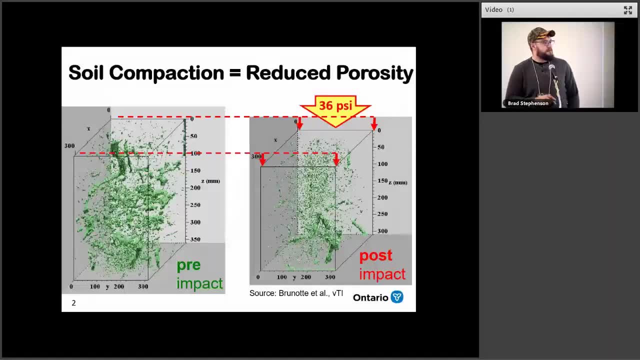 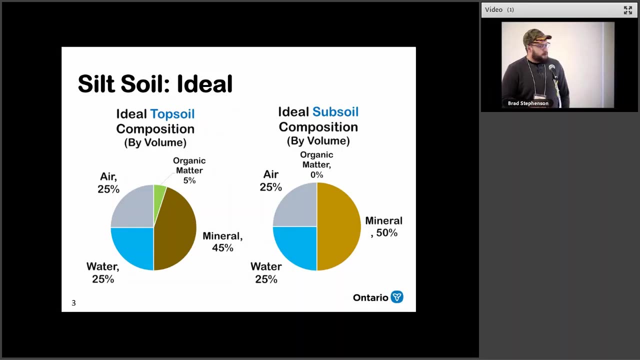 give extra real answers. you want a 50% void space. so you, if this, if you sort of math all this out, you'd want about 50% void space for an ideal soil sample, 50% green area there and that's for air and water. it's not always 25 and 25. 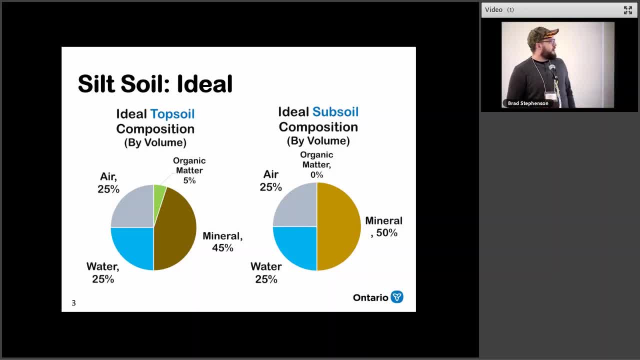 sometimes it's wetter, sometimes it's drier, depending on the time of the year, and we'll get into that a little bit more. but half of that space in that volume you want for air and water, that's where everything happens. ion exchange, all your nutrient uptake and root growth and worm worm traffic areas, that's what you. 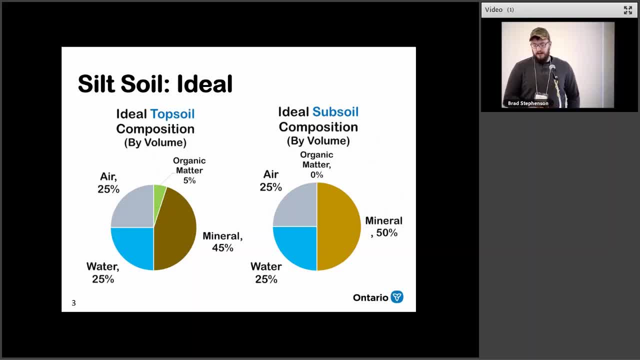 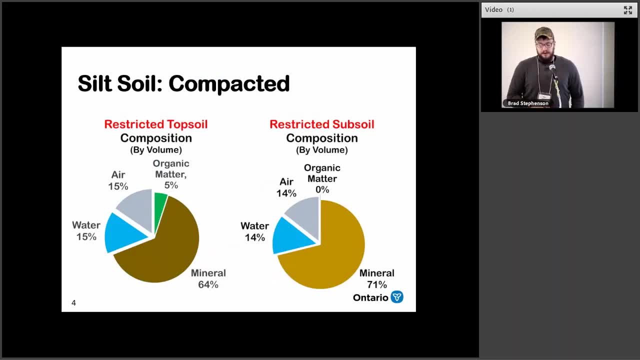 want now, when you get to a compacted soil and it doesn't take much to get to a point where you'll see reduced root growth, so, or reduced crop, poor crop in general, so not too much. so only a reduction down to about 30%, and now we're definitely into some restricted, restricted growth. 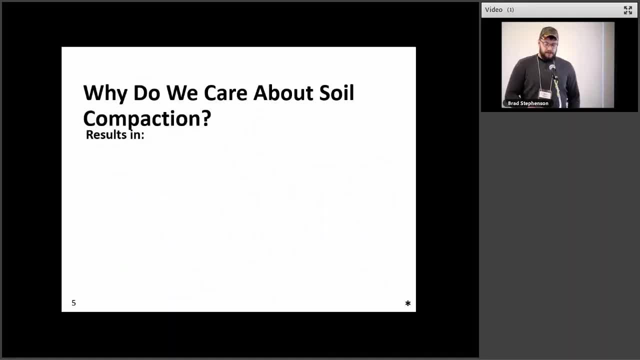 conditions. so why do we care? so I've kind of alluded to it and you might know this: decreased water infiltration, reduced holding capacity. so if you get a big rainstorm, if you've got no void space for that soil to take up water, it's not gonna hold any. you can think of it as a 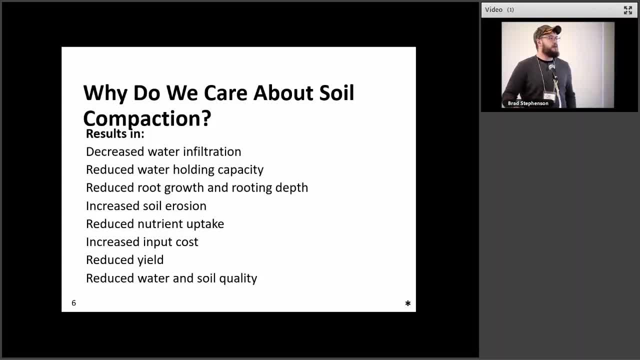 you go to any parking lot in any strip mall, anywhere underground, under that parking lot there's a bunch of empty culverts all tied together in a network and it's to take all that rain event and put it somewhere and then get rid of it when it's not raining, when you can, so you can think of your void space in your 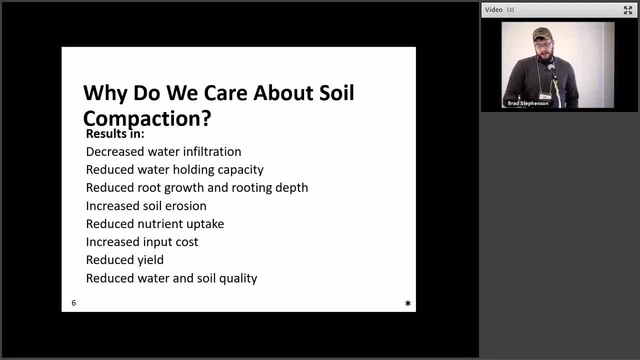 soil sun, kind of like that capacitor in your soil. you have less of that. if you have less of that, you have more over land flow, which means more, more soil erosion, again reduced nutrient uptake because you have less space for nutrient uptake to happen and reduce real yield and poor water. 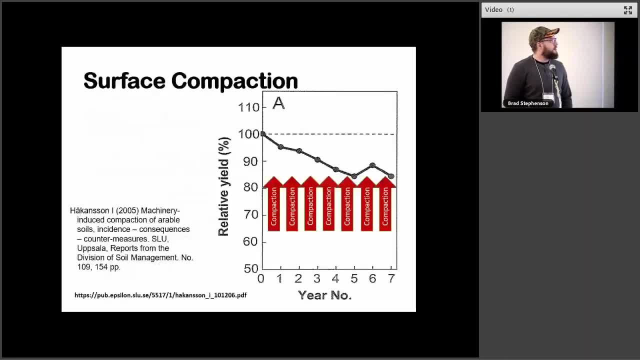 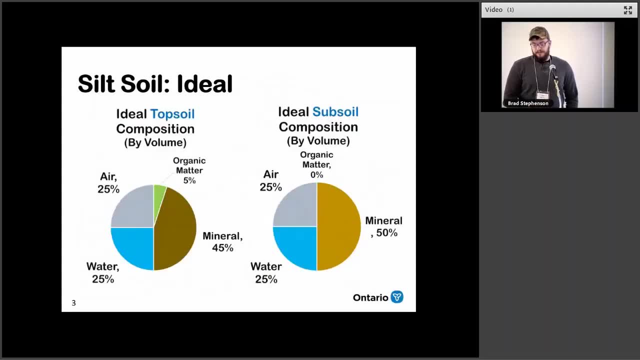 quality, so on and so forth. so I'm preaching to the converted. probably compaction equals bad, but that was just the topsoil. so if we looked down at subsoil, what's the major difference between topsoil and subsoil? yeah, organic matter. so the organic matter acts kind of like fiber fill and your 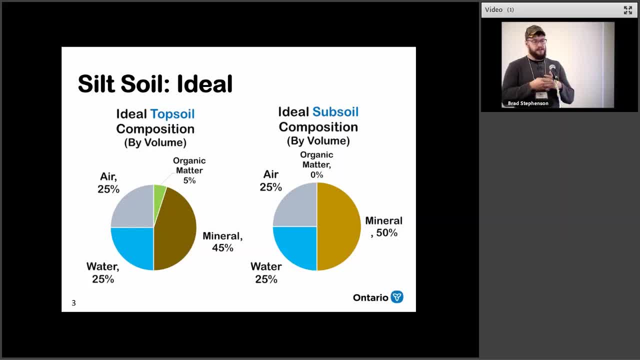 concrete mix it gives. it gives that top soil a little bit more tensile strength. so if you can think a little soil particles touching each other, if you've got organic matter weave throughout that profile, it's going to be generally stronger. so in the subsoil, subsoil, without that, you know organic matter or 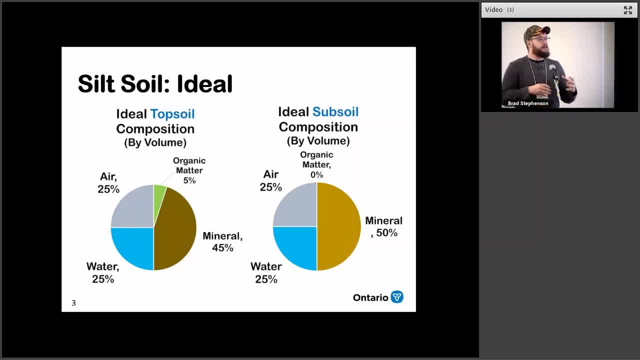 all those that root mass or organic mass. you're gonna have a little bit weaker soil so you can picture it as a really good mattress on top of a really poor mattress. so you can be comfortable on the top mattress. but if you're heavy enough you're gonna squash the bottom mattress. so we'll get into that a little. 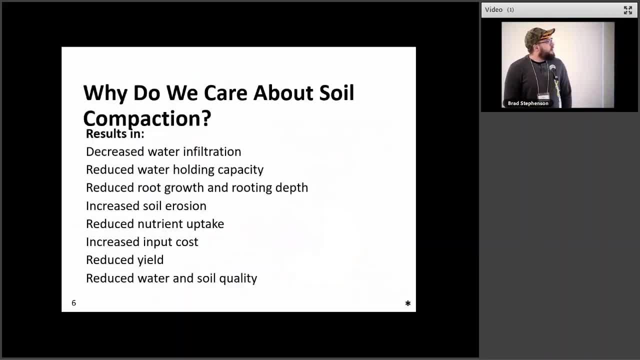 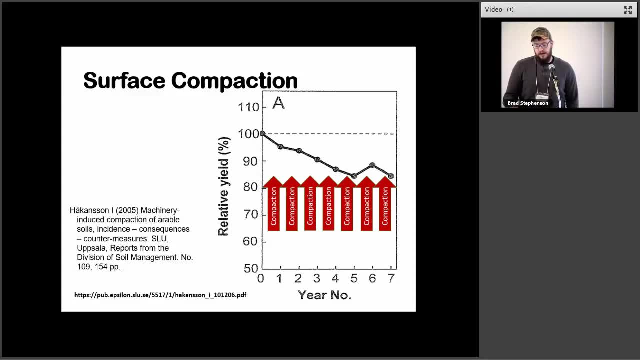 bit more, but you can kind of think of that as we go along: subsoil surface compaction. so this was a research done many, many years ago in Europe somewhere, but they did a compaction event every year and then they did a survey, and they did a survey, and then they did a. 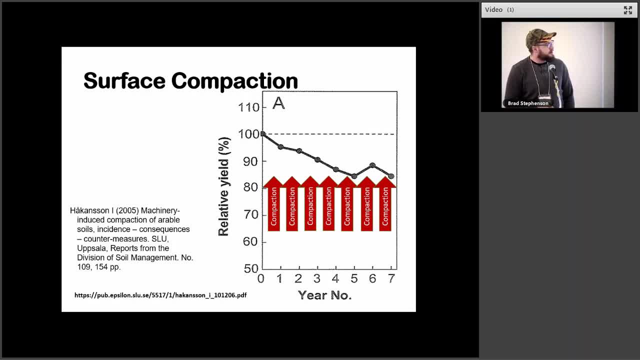 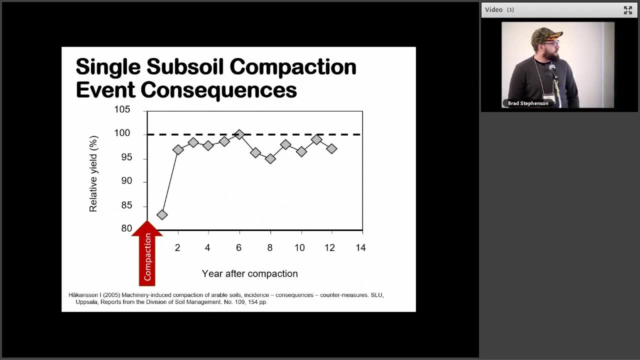 for seven years. so they compacted it and you can see the effect of yield. yield percentage is cumulative. so every time you compact that, every year it's a little bit more cumulative and it does rebound. so here's a single compaction event and then followed by the yield after the years. 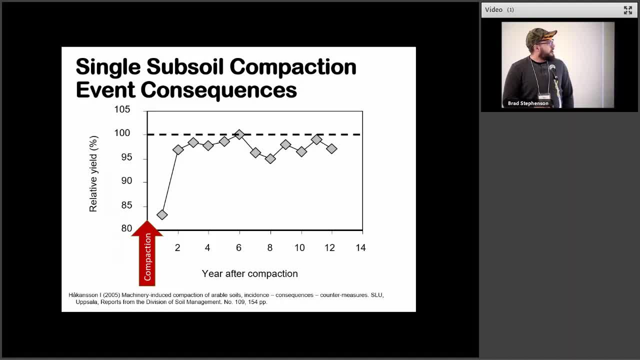 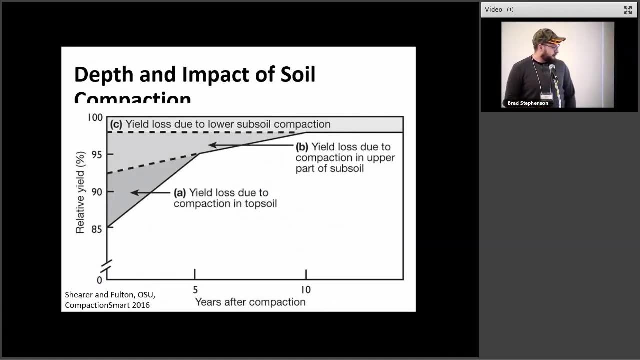 after that and they did quite a bit of study on this but it never did get back to 100%. there's about a 3% permanent loss from compacted soil after a compaction event, so it is cumulative. so again, this was done by this, one was done by sheer Fulton and OSU and it kind of mimics the same. 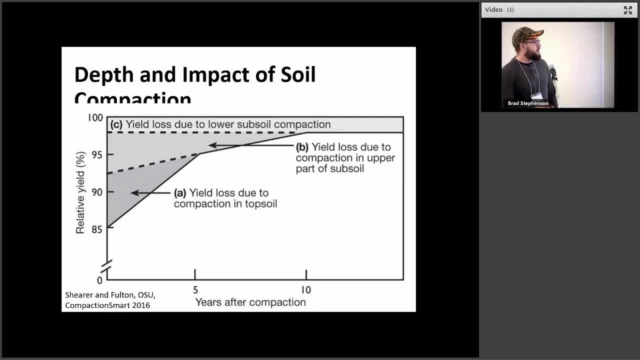 thing. so in the first year following a compaction event you see an immediate reduction in yield percentage. so 100% being you know what you would expect. you see your immediate reduction and then in the years after it does recover. so this would be the topsoil compaction. so that's the stuff that we can kind of take care of with. 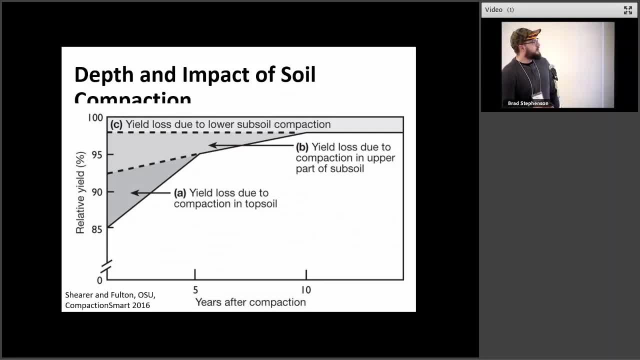 good management practices. due to the, the upper part of the topsoil again a little bit harder to till, a little bit harder to work kind of hard to get organic matter down there. so it takes a little bit long to recover. but then in the real deep stuff, the deep compaction, you do get that permanent loss. 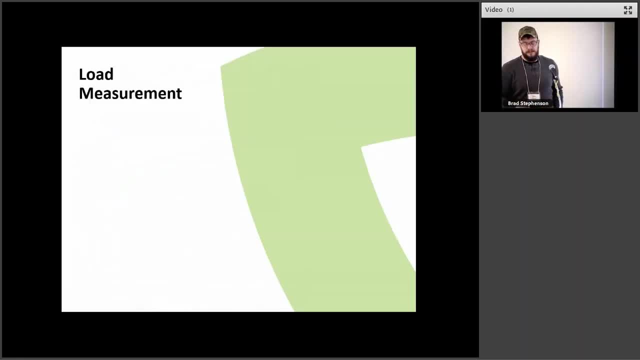 and that's probably mostly due to poor water infiltration through that profile. so when I say we wanted to compare tractors and tires and different axles and different configurations and everything under the Sun, we needed a way to do that, so we borrowed this method from Matthias. 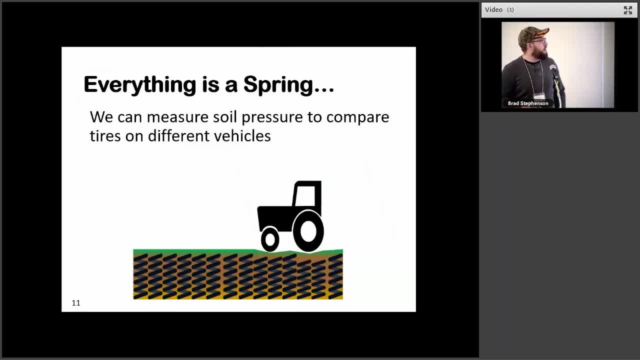 when he came over, but you can again think of everything like a spring. so if we measure the pressure in the soil, that'll give us a good indication of what that soil, what load that soil is, you know, experiencing. so you can think of your, your soil profile as one big giant. 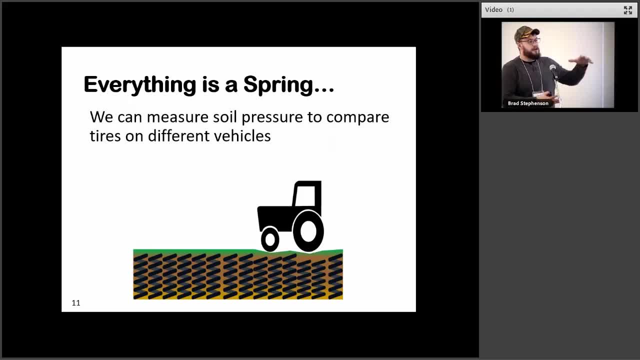 spring. of course, if you compress a spring it has to move. if you move that spring a little bit too far, it won't come back to its- you know- original state it'll. if you exceed the yield stress of that material, you will permanently deform the material. so I've trimmed out a bunch of the slides. 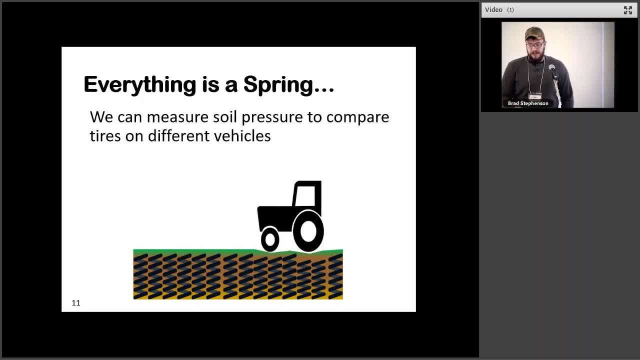 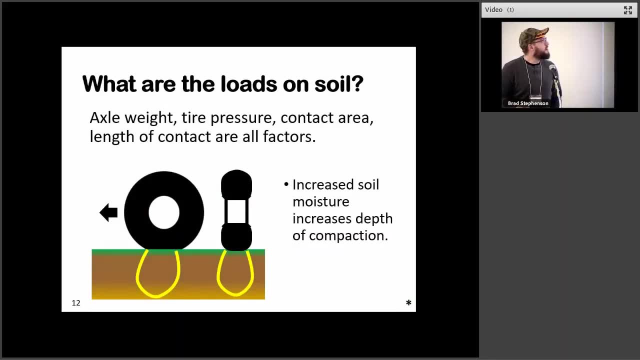 here. if you have any more questions about this, please do ask. but you can think of the soil of the spring. if you push the spring a little bit too hard, that's probably a bad thing. so all the factors that go into this are the soil that you're using. so you can think of the soil that you're using. 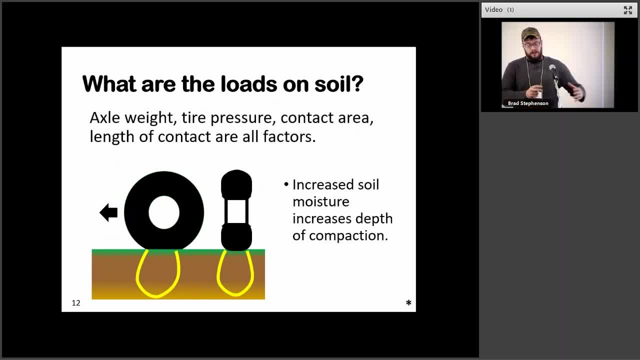 this: axle: weight, tire pressure, the contact area, the length of the contact area, the width of the contact area and then again, if we're talking in generalities on soil, we can say that yield stress is about 15 psi. but if you have more organic matter or less organic matter, or more clay, more 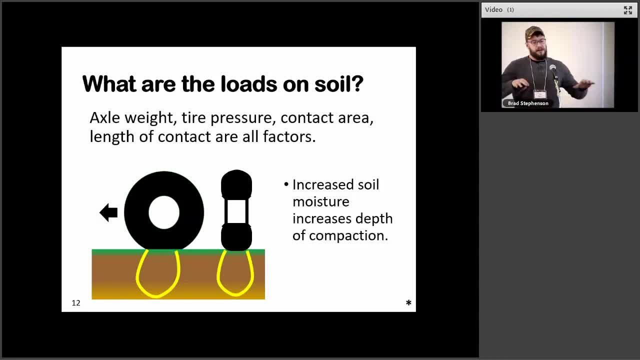 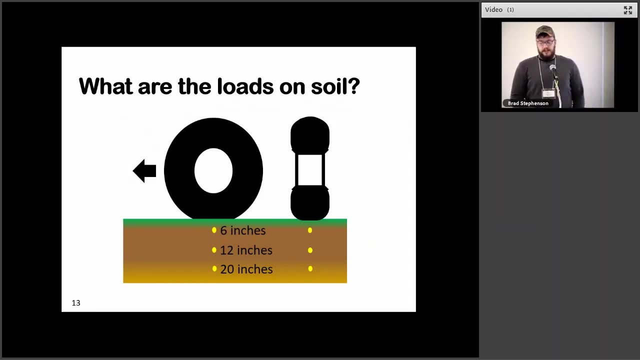 sand, higher moisture, whatever that move of that, 15 psi is going to be a moving target. so yield stress is going to vary quite drastically and that'll be important when we talk, when we consider things in the forage system, I guess. so we compared stress in the soil for all these vehicles at 6, 12 and 20. 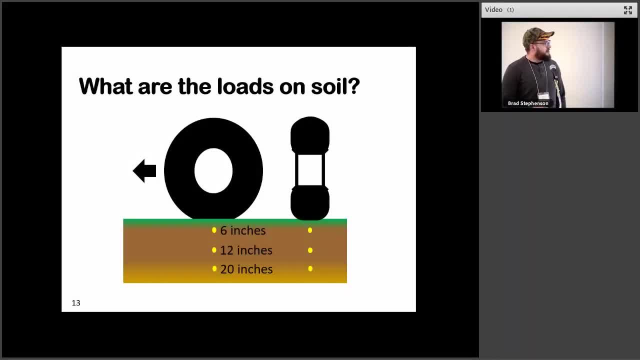 inches. so we're doing that topsoil layer sort of 16 and 6 inches down, just kind of out of the way. obviously, if we laid it right on the surface we'd, you know, just be driving over a bare sensor after a while. 12 so sort of, at that interface between topsoil and subsoil, topsoil and subsoil, and then 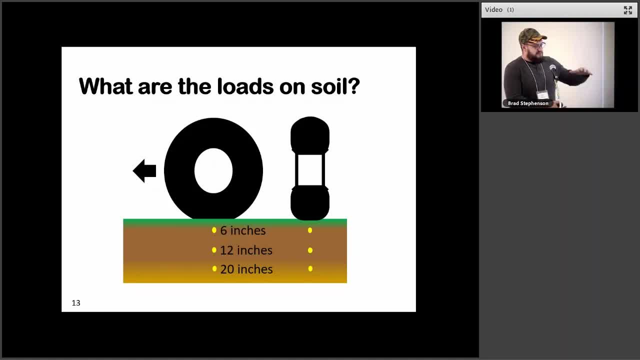 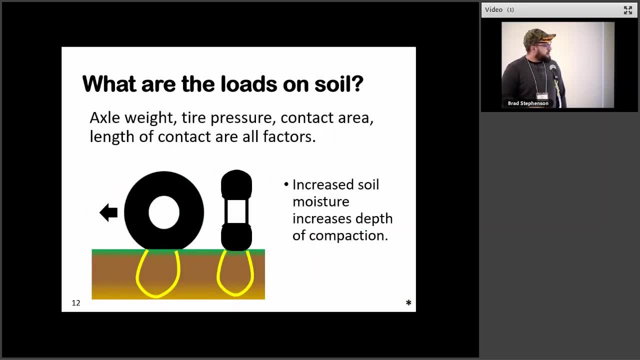 20 inches, which is just a good depth that you can still see some of the loads. so the load you can figure sort of dissipates into the soil a bit like a balloon, so you get kind of a bubble. so as you stress that soil the affected. 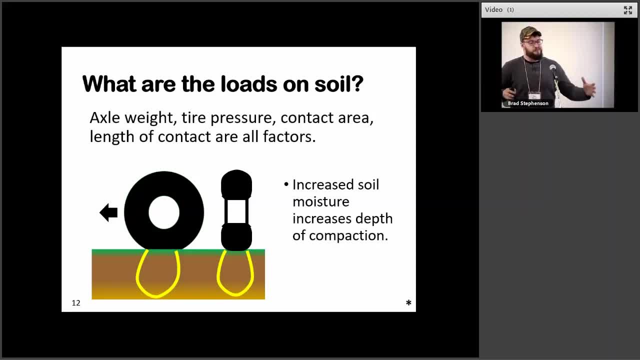 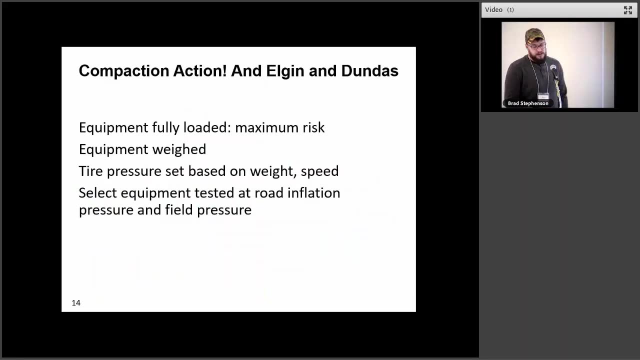 area in that soil is kind of a bread loaf or an inverted road cone kind of shape underneath that soil or underneath that tire, under the contact patch. so that's what we're measuring. we're measuring sort of a point load inside of this stress bubble. so when we did these compaction events we did we had a whole whack of equipment, so everything that. 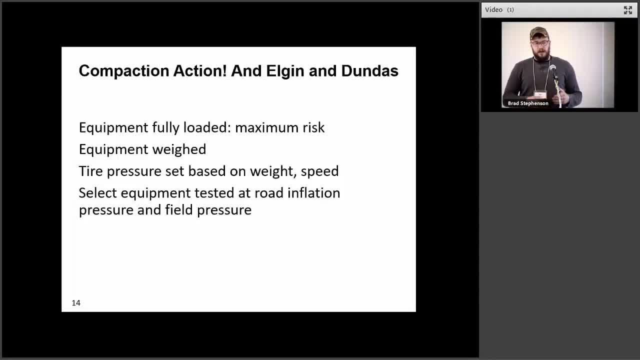 all the neighbors could think to bring, and we loaded everything up to their maximum weight carrying capacity, sometimes over, if the manufacturers would let us in some situations. we weighed all of the equipment on individual tires. we set the tire pressure based on the weight and the speed of travel on that for that vehicle. so what you would expect to set the tire pressure to. 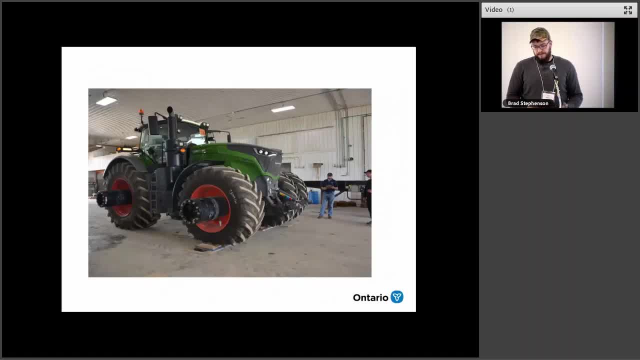 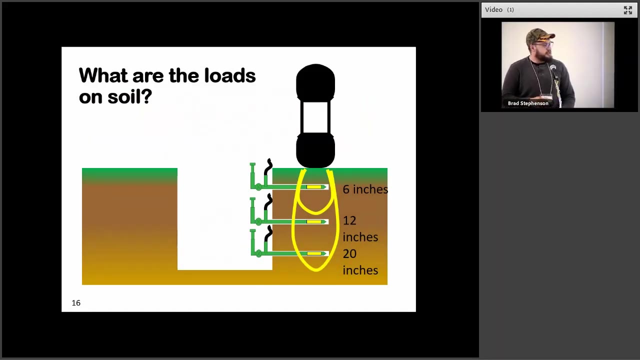 safely carry that load down the road or in the field. so in this case we had a Fent Tracker, we got pad scales. we're measuring the, the individual weights on each of those tires so we can measure our load and, like I say so, the soil, the pressure sensors. basically it's a rubber balloon filled. 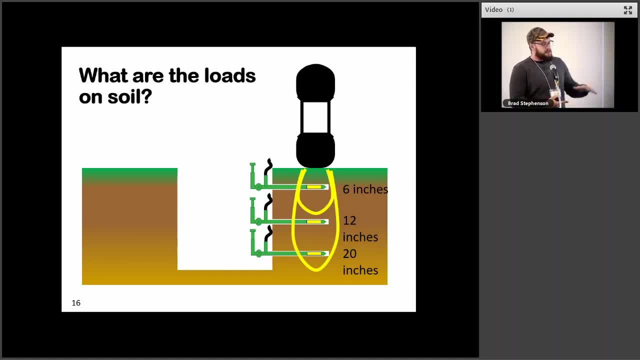 with water. I have a pressure gauge on the end stick that in the soil. you need to drive over it. you get a pressure inside that balloon that you can measure and that's what we're using to compare all these visit vehicles and the stress in the soil. so a little bit of some of the examples. so here we have a. 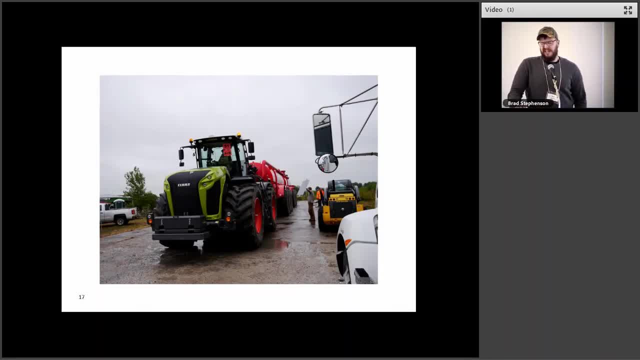 manure tank. this one was the probably the most uh visual effect, I guess, on tire pressure. so that's a Clausier on tractor with a noon quad tank, 110 000 pounds gross. uh, traveling through the field on eight axles. uh, so we have the our setup in the field. uh, this was on one of our test days. 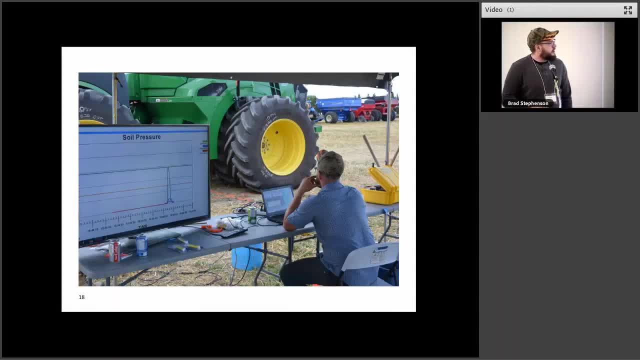 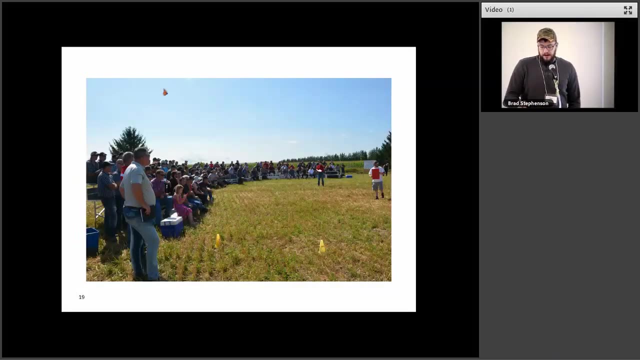 over in Dundas. I've got all my little sensor rigging. we have the soil, the sensors in the ground over here and we're driving vehicles on it and I'm frantically saving data to a file, hoping that I will remember what I did two months from when I was sitting there on the Thursdays we usually do. 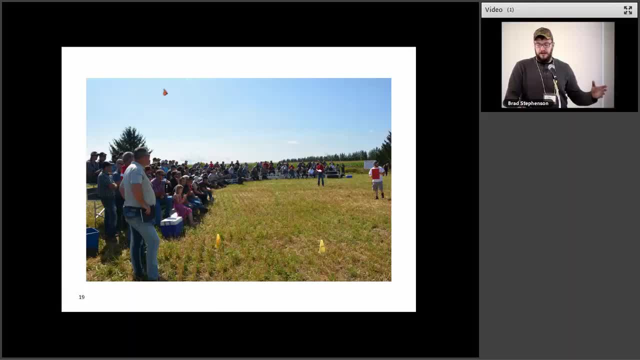 a Monday, Tuesday or Tuesday, Wednesday, Thursday for these events, first, two days of research and getting everything organized and weighing everything and making sure we've got all our ducks in a row. on Thursdays we do the live demos, so we drive the most interesting vehicles over these sensors while 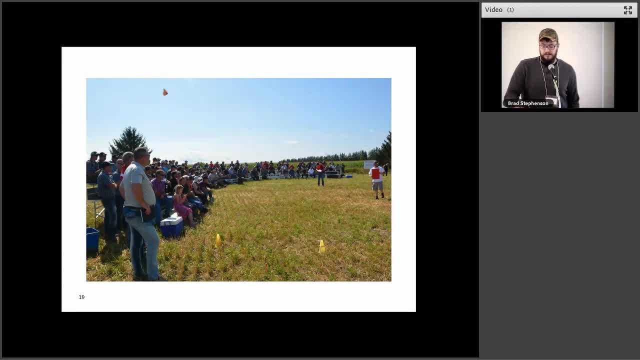 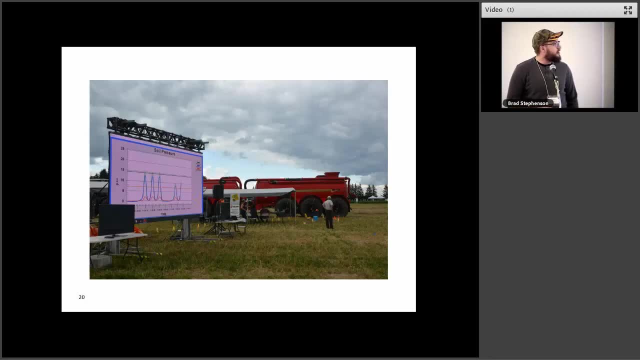 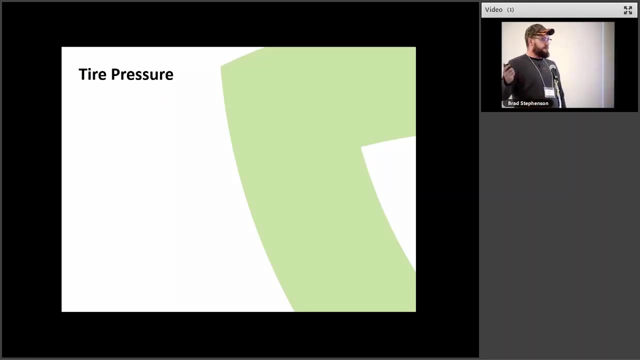 there's a crowd of 150 people watching me to not screw it up, so we had a big jumbotron. this was out in Dundas, so you can see these plots being created in real time and that's usually pretty awe-inspiring. so what's the big deal? I mentioned so this tank. again, this is about as most low, as much load as you. 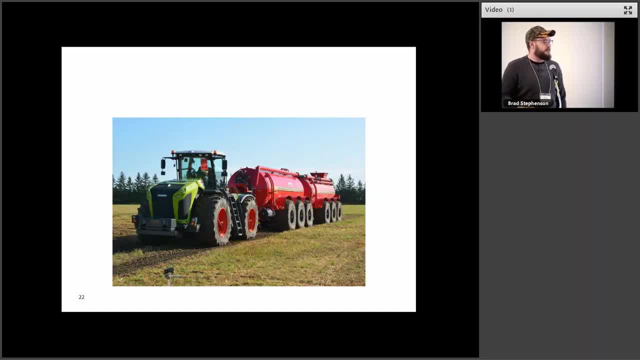 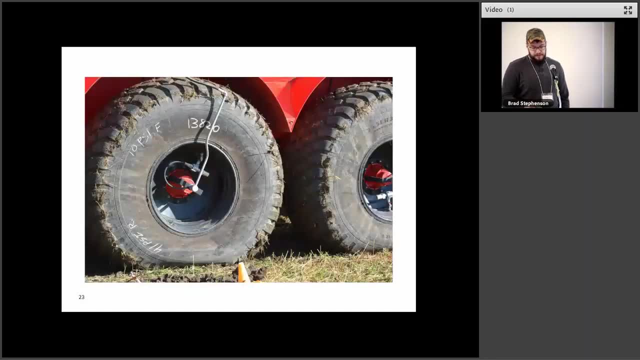 can put on a hayfield and and more and on the livestock. if you've got livestock, uh, you might do the thing where you work. there we go. so this vehicle, about 13 000 pounds per wheel, uh, on this vehicle, so both sides, uh, and that road pressure to carry that load down the road, you have to be at 41. 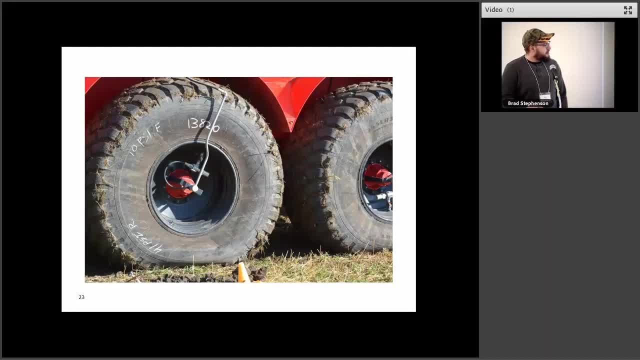 psi. uh, with these tires you can see how this tire is squatting, uh, increasing the footprint of that tire. uh, when you slow that speed down from road speed down to field speed, you can get that tire down to 10 psi. so this vehicle had a central tire inflation system so that you 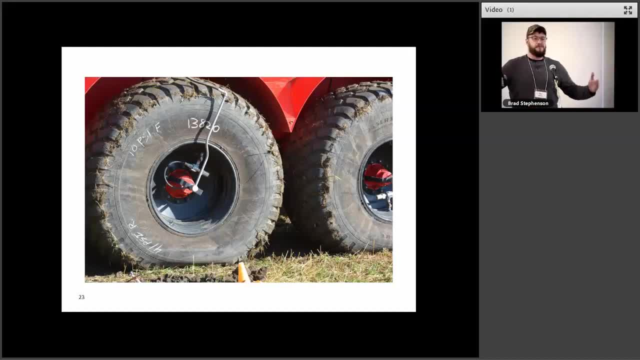 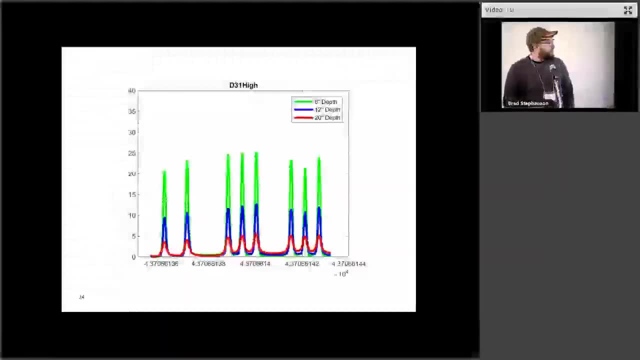 can make sure that your tire pressure is always at the the most optimum tire pressure for each condition. and here's kind of the plot. so this one's a little bit more intuitive than the other ones. so this is time across the bottom and my vehicle is driving, in this case, I guess. 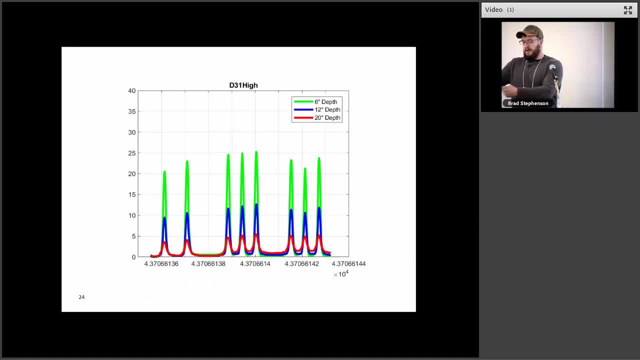 the right um over the sensor. so bang, bang, bang, bang bang as each axle comes over that sensor. so this would be the front axle of that vehicle, second axle of the vehicle and then each of the axles on the tank. so what this tells me? this vehicle is pretty well balanced across front. 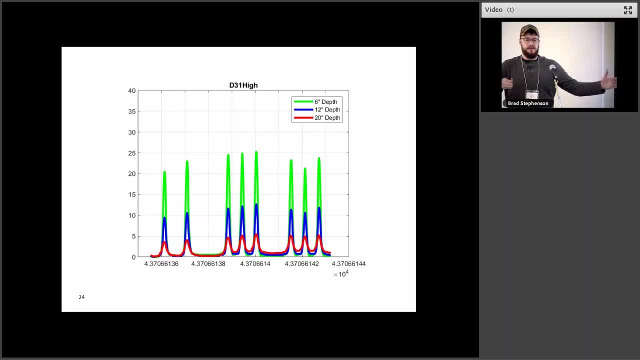 to back on that, uh, that whole setup. so there wasn't one axle that was carrying any more load disproportionately. so that is a factor when you can consider setting up your equipment, but we're still going to be in that area where we're going to be causing compaction. uh, the 12 inch depth- same. 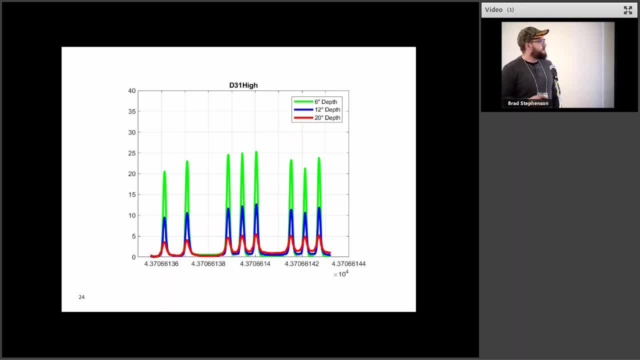 story: uh 10 psi and the top soil layer. so you remember what I said was yield stress for a an average soil 15. so we're definitely in the realm where we're going to be causing some amount of compaction in that top six or eight inches- again, condition dependent, but for most uh good. 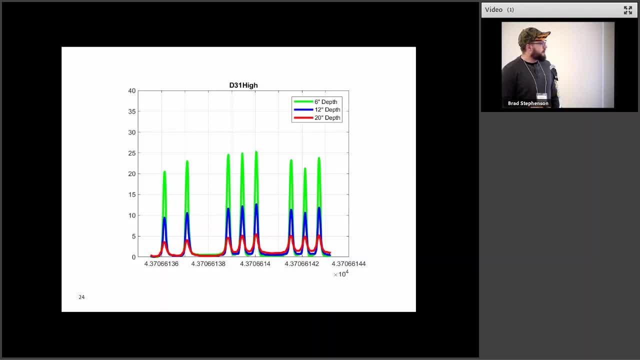 conditions on decent soil, we're still going to be in that area where we're going to be causing compaction. uh, so we're getting pretty. we're still at 12 inches. we're still at a risk of causing some compaction, even though you may not see a rut on the surface. uh, and then at the depth, watch when. 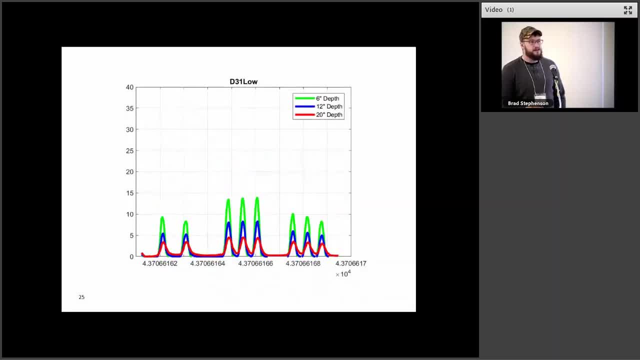 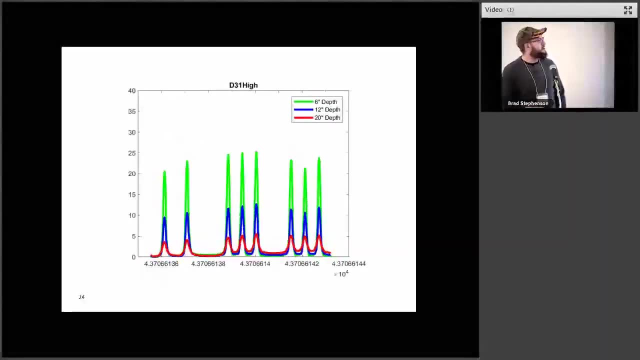 I flip through these graphs left and right. is that red line change very much at all? but you see, the top two lines are changing pretty drastically. the scale on that grasp isn't changing, other than the fact that the, the actual size of the picture, is changing. but when I reduce that pressure. so this: 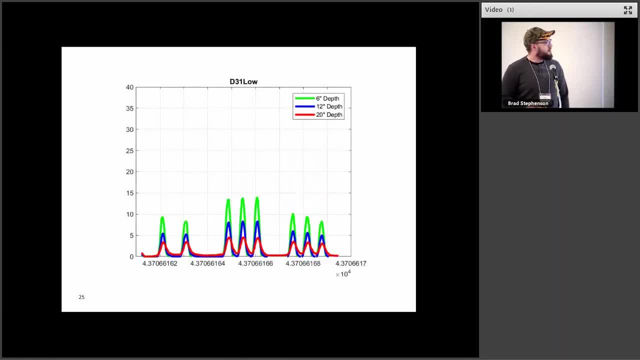 is now at the low pressure. this was at one psi, this is at 10 ps, or, yeah, 10 psi. we've drastically reduced that, uh, that top soil stress in that soil profile. so now, if we're on a good, a decent soil here, now I'm probably not so much. 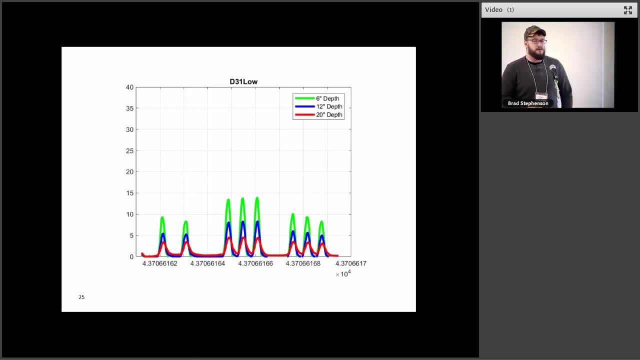 concerned about compressing that top soil layer. so that was a real big, dramatic impact. and this was one of the most obvious ones when you get it in the field. and it's more interesting too because the sheer amount of weight on that vehicle- uh, there is not enough tire, or. 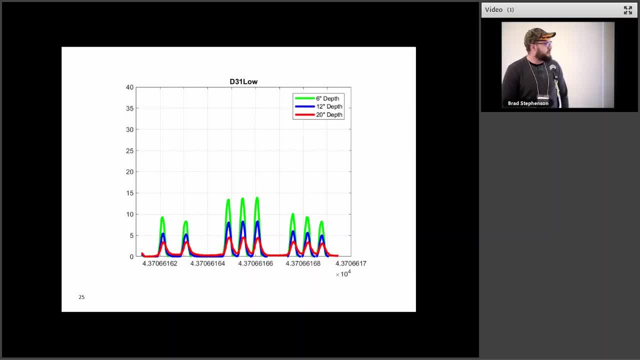 low enough tire pressure that you can put under those axles and expect it not to crush. uh, the 20 inch layer. see, Greg Stewart has a good analogy for this. if you've got an old wooden trestle bridge, and I take my pickup truck with narrow tires, high pressure and drive over it and falling through, 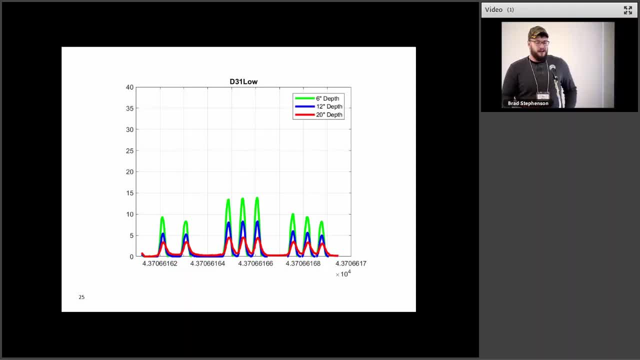 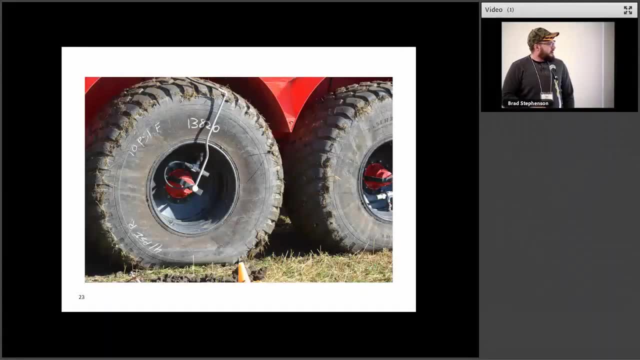 boards and cracking all the boards and the decking and falling through the decking. but I'm going to get over the bridge because I'm not very heavy. I can take my big manure tank with my low inflation tires and that might not even break a part. but I'm going to get to the top of the bridge and the whole bridge is going to fall down. 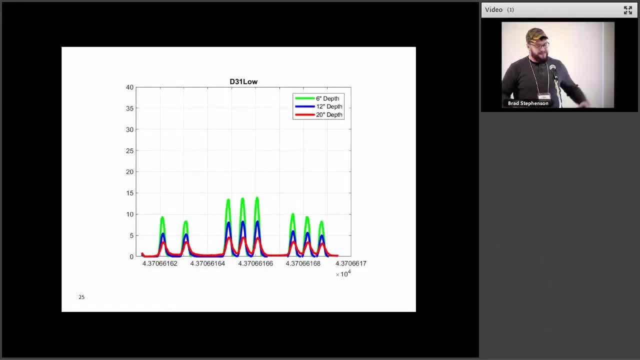 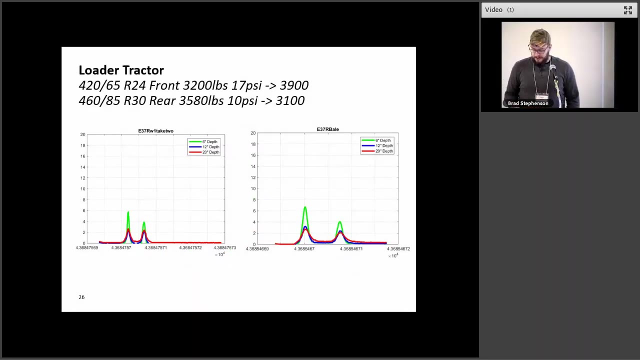 uh, so you can think of the top soil. stress is that, um, there's just a massive amount of weight pushing that whole, you know, area of soil straight into the earth. uh, that that depth is still going to feel the magnitude of that weight. so that's going to be important when we talk. I'm going to talk specifics. 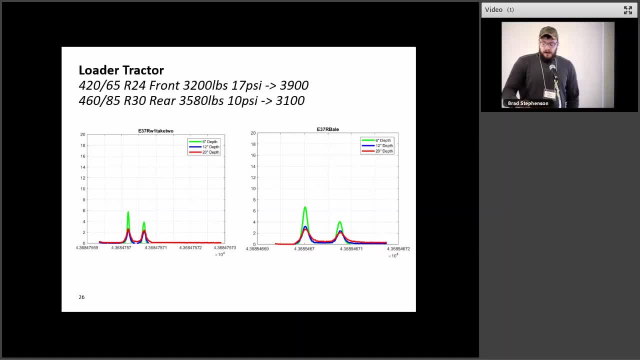 about Forage equipment, if I can do it in three minutes. uh, here's another interesting one. so this is a loader tractor carrying bale. uh, this was on the right hand side. we had a pretty decent tire. this was, I think, a VF tire, uh, 17 psi in the front because it was doing loader work, so a little bit higher than what. 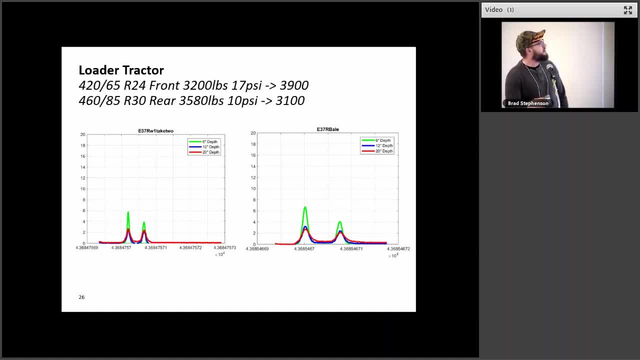 you might normally expect. you put a uh empty, driving around 3200 pounds of the front. you put a bale on it, you increase the rate to 3900 pounds, uh, and there's the response we get. so a little bit more response, or a little bit more stress. I guess with the bale there's only a. 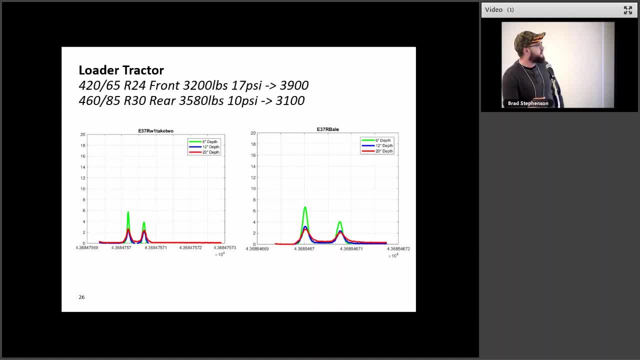 what a 600, uh 700 pound difference there. so not not too much, uh. but then compare that with the narrower front tire on the other side. uh, we had a narrower tire with a lot higher psi. our response in that, um, topsoil stress was was quite large, or quite a bit higher, I should say. so, um, comparing. 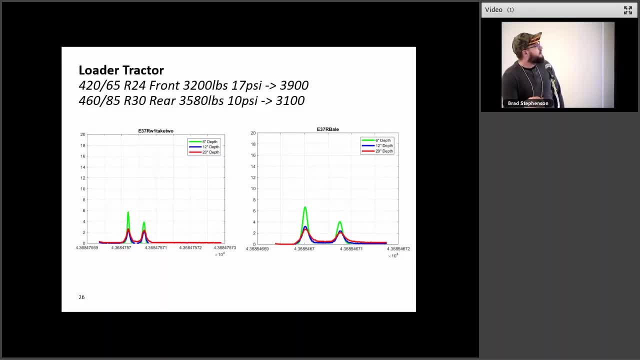 those two situations: a better tire with a little less uh psi in that tire, uh, and then you get a lot higher. uh, really benefited, benefited me, benefited me for the exact same vehicle so I can, you know, more comfortably drive that across my field. um, I guess, in that situation, 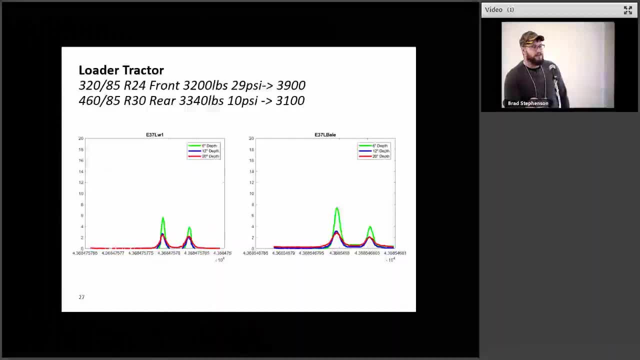 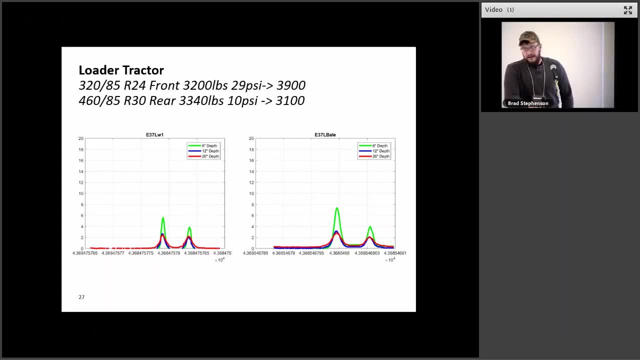 uh, any questions? up to this point have I totally lost anybody um on the internet. you can just call Brad um. so that's what we're doing and I got a whole whack. I think I got uh 60, some odd scenarios now, plus well, plus Arthur, so getting close to 300 scenarios. 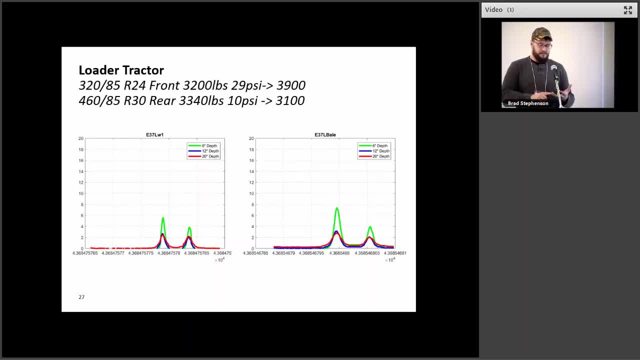 um that I can sort of amalgamate. I'm going to have tire load pressure um tire size, so I can see if there's any. is our big tires generally better, uh, all the time, or is it more of a function of psi? it's probably more of a function of psi. so if you take anything home, 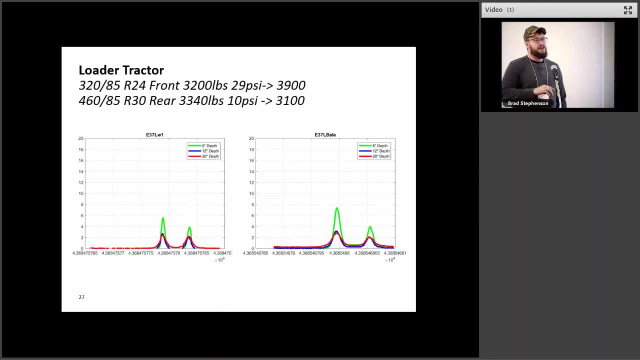 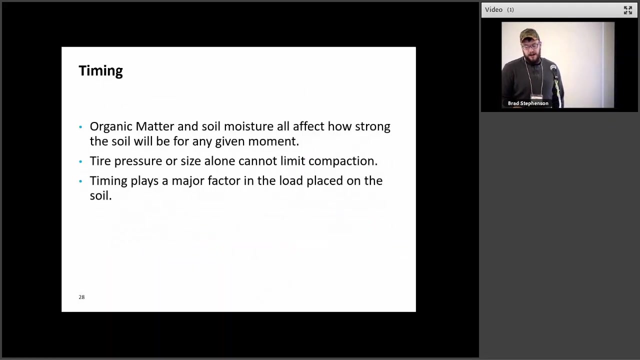 from this, less pressure is better, uh, for most cases now, you still have to care, carry the load safely, uh, tire warranties and such and so on. uh, but generally if you're in the market for new tires, uh, you have a choice between two tires. the one that will carry the weight at lower pressure is better from a compaction standpoint, uh timing. 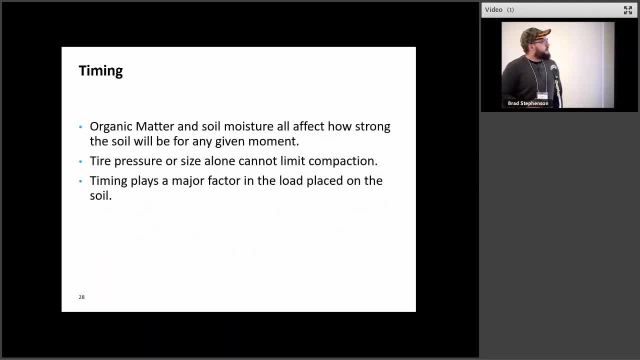 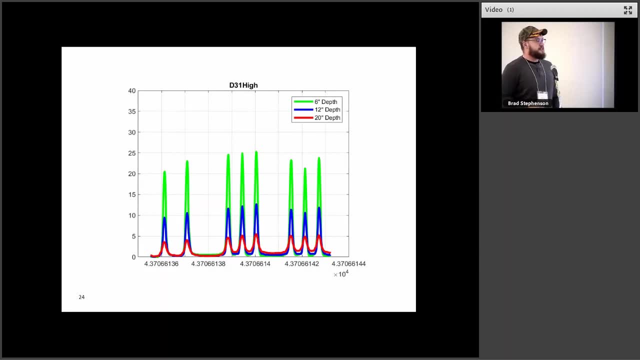 so I mentioned timing. organic matter and soil moisture are going to affect how strong that soil is. so again back to this: if I'm on a hard dry clay, psi isn't going to touch a hard dry clay. we make houses at a hard dry clay, um. so on a wet clay, though, that's very much guaranteed to cause some issues again here a. 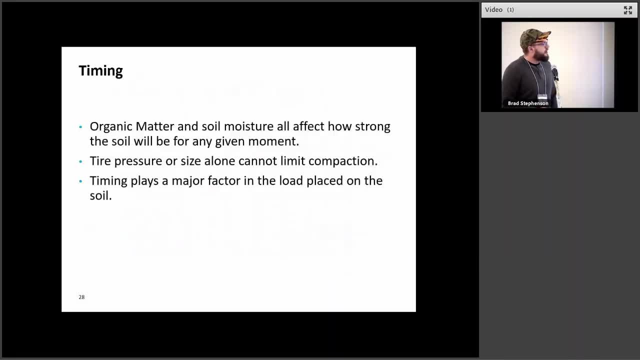 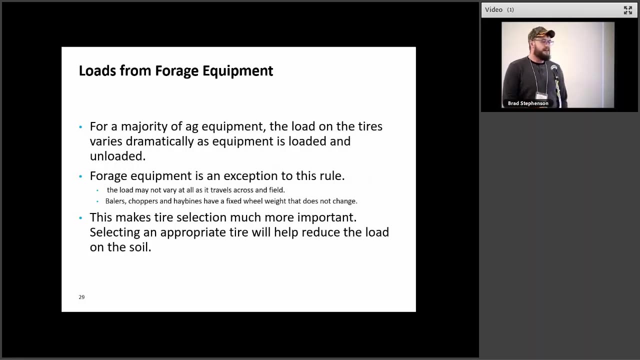 wet clay probably not going to be strong enough to hold that load up. so timing's a big thing and tire pressure and size alone can't limit compaction. you do have to still be kind of strategic with when you drive on stuff. so timing is a big, big factor. I realize that any calendar 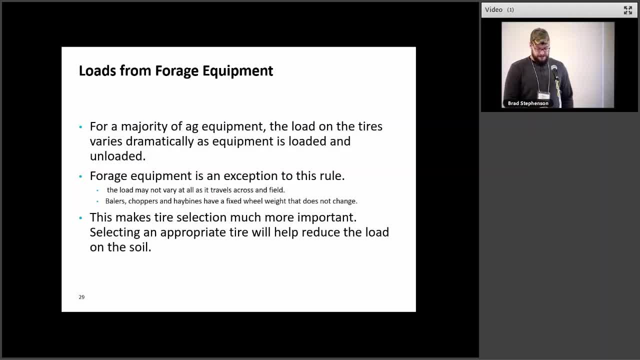 in system that forage is. timing is not always beneficial, especially if our last speaker was saying it was getting too tall, you better cut it. well, if it just rained, probably not an ideal time to cut. for the majority of Ag equipment, the load varies pretty drastically, so that manure tank I 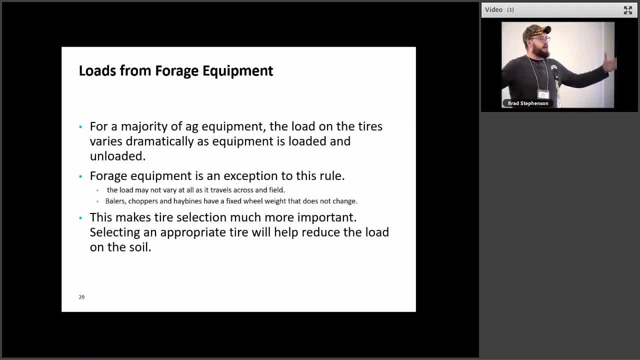 said it was 110 thousand pounds gross. it's not always that because you do empty it at some point, you go back and get more. so at some point in that field that level of risk drops down to a reasonable level. with forage equipment, though, forage harvesters, the same weight all the way. 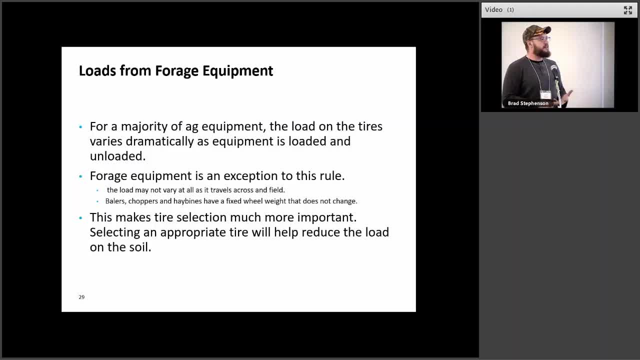 across the field. balers always have two bales in it, same weight all the way across the field. so in most cases, uh, the forward equipment really doesn't change its weight very much, so getting the right tire pressure on that vehicle is going to be really important. uh, Baylor, uh, the entire selection. 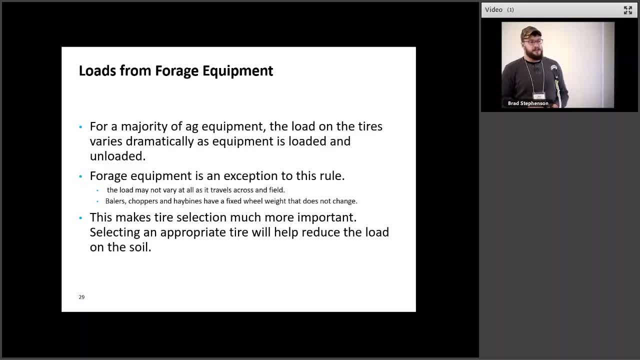 so I've seen a lot of balers in the last two years that had bias ply tires on them that are over about 45 PSI. it's not really doing it for me in most cases, so if you have the opportunity to replace tires on your baler or you're buying a new baler or new forage equipment- whatever it is- it could be a. 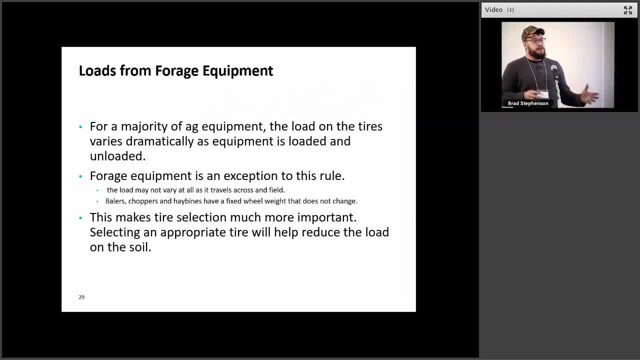 wagon could be whatever, putting some thought into that tire and getting that tire pressure reduced. either go into an IF or a VF tire, something that's a little bit more conducive to lower pressures for some weight. but that's an opportunity where money is not going to be wasted, I should say. I guess I 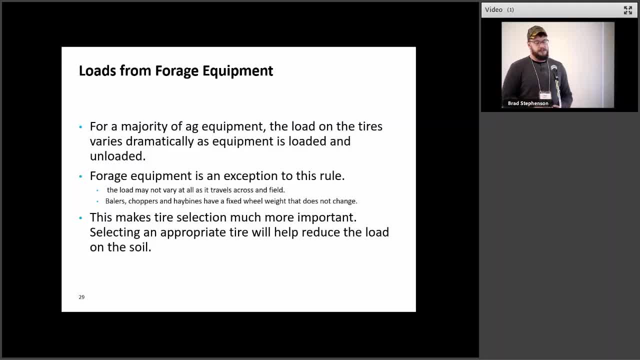 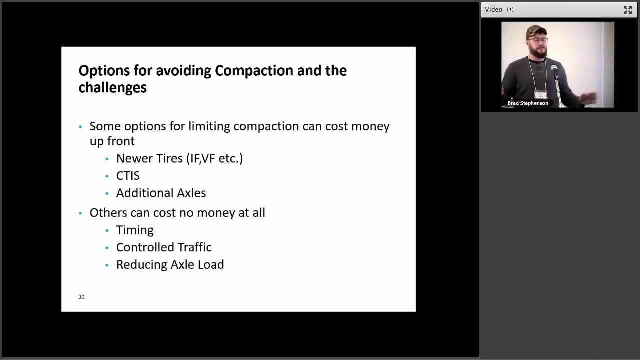 can say, um, putting a better tire on those pieces of equipment, uh, the options. so, uh, there's basically there's a whole bunch of stuff you can do in a from a management point of view, you don't have to throw money at the compaction uh problem. but if you do throw money at it, you're probably going. 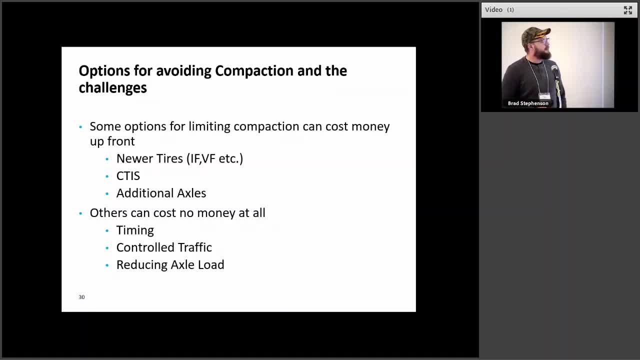 for, like I say, newer tires. so the IF increased flex, or VF very flexible, uh, those are tires where the sidewall actually takes up a lot of the effort. um, in a bias ply tire, you rely on the air pressure in that tire to keep it as a as a you know not. 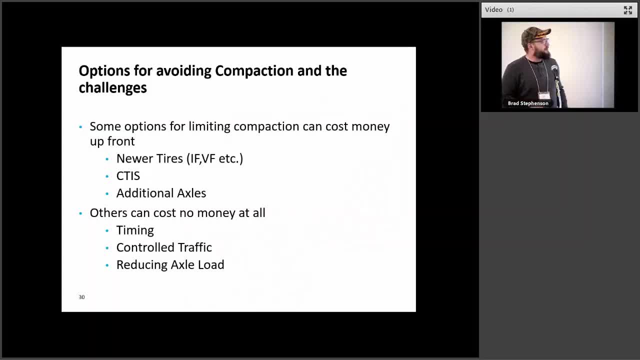 fail to make sure it doesn't fail, and a VF or an IF tire. it's not so reliant on the, on the PSI, to make sure that system stays together. so the, the tire itself is better at at holding itself together, um, or you can go to a central tire inflation, so you can sort of take the, take the human element. 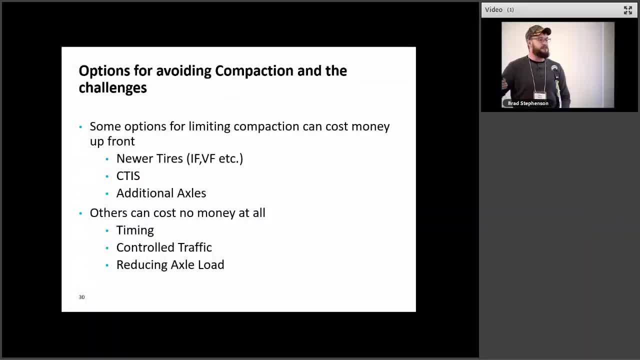 out of it. you still have to do your homework and figure out what your tire pressure needs to be, but now, when you pull onto the road, you can pump the tires up and you don't have to worry about it. um, and you don't have to drive around with high pressure tires all the time. one thing I am looking. 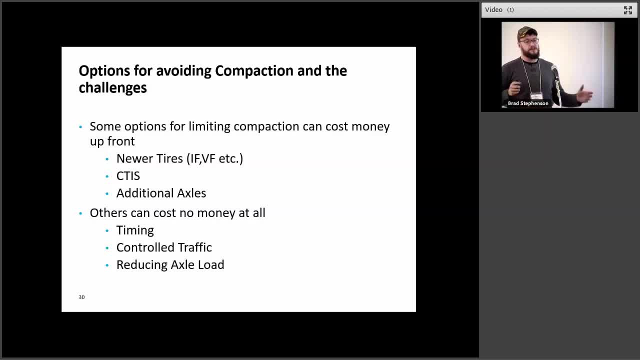 to do in the future is do some live fuel efficiency demos. so pulling a high inflation tire through a field burns more fuel. you're always trying to pull it. if it's sinking into the ground, you're always trying to pull it up out of that rut. so you're going to burn more fuel. so I'd like to kind of 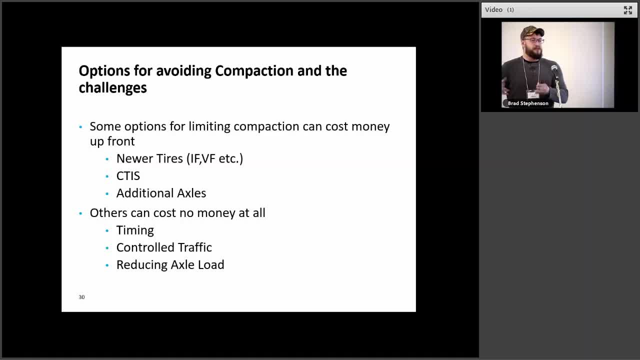 structure, um, to the other end of the spectrum, and how can I save money just by having a proper inflation? uh, and then, like I say, if you're in the opportunity to, if you've got the opportunity to replace equipment, thinking about more axles is is always a good, a good time, so you can think of it. 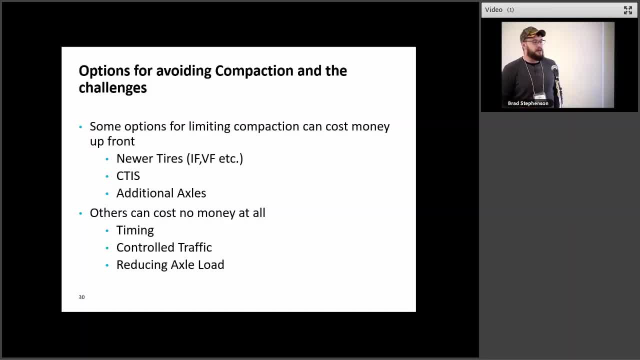 as that, uh, that total weight or that total load on the soil. reducing that load is going to be better. uh, some stuff that costs you no money. I don't know why I put controlled traffic down here, because I wanted to kind of, um, uh, what's the word, without being rude, um, controlled traffic is going to be difficult. 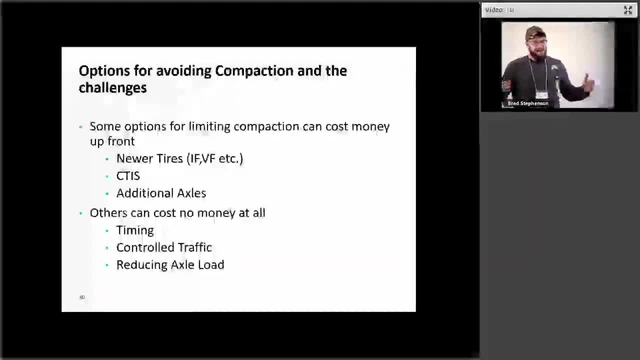 uh, in a forage system, because uh controlled traffic, you really need your vehicle widths or your implement widths to be all the same so you can stay on the right tracks. um, if you're cutting hay eight feet at a time, you're not going to bail at eight feet at a time. 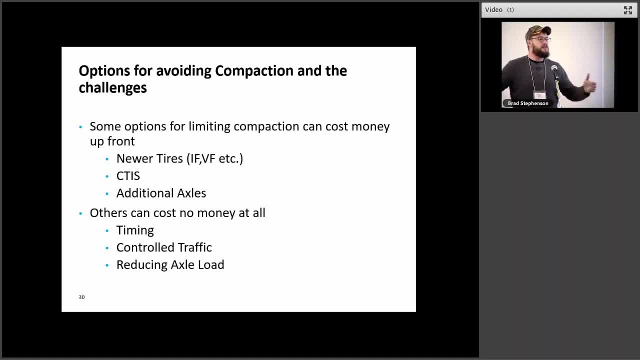 well, maybe you will, but it's really hard to match up track widths at that point because you get, and if you're in a custom operator, if you're hiring custom operators in, they're not going to know where your tracks are and it's going to be a real management headache to go to controlled traffic. but timing and reducing your 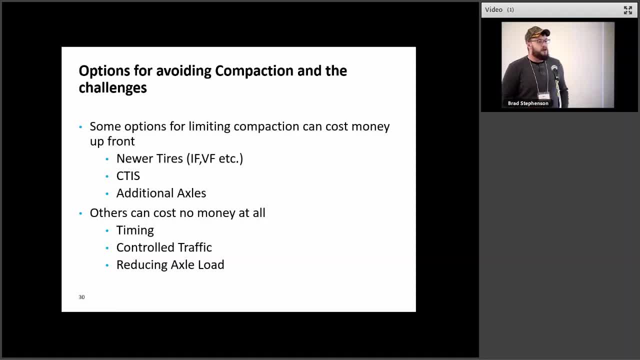 axle load. so being kind of strategic about where you're driving and when you're driving in the field, don't start on the wet side of the field. if you can go to the dryer, better soil and through the day, because even in about six hours you can really drastically improve your soil strength. if 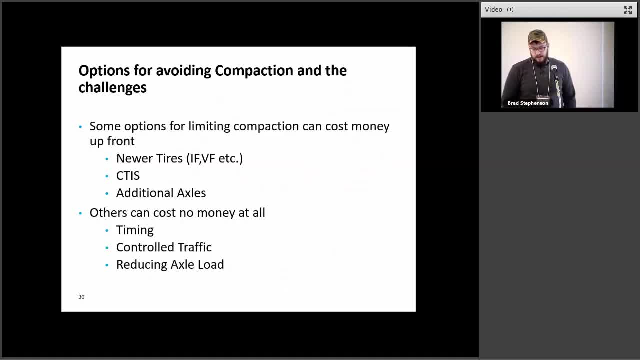 you've got a good, uh, a good day for hay. the same rules apply for soil, so, uh, with that, we'll quickly do some questions. I got six minutes for questions, so so most of the talk online here was about how- how we're going to fix the Toronto Maple Leafs and, uh, they weren't really 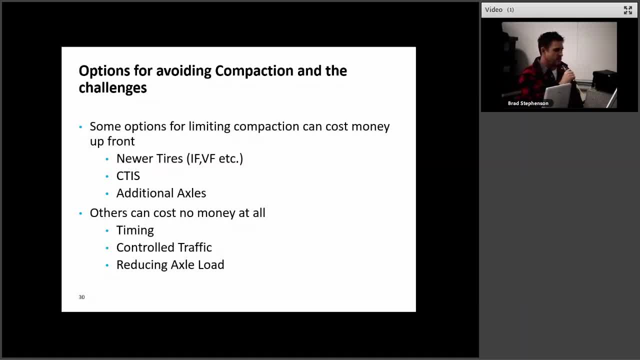 paying attention to your, to your talk, Alex. but uh, we, we all agreed that, uh, the number one move is to sign Alex Barry as their backup goalie. so we got that one solved. confidence is is bad right now. your confidence is, my confidence is battery. no, it's not. but then there was another question. it's, uh, how do we go about remediating the? 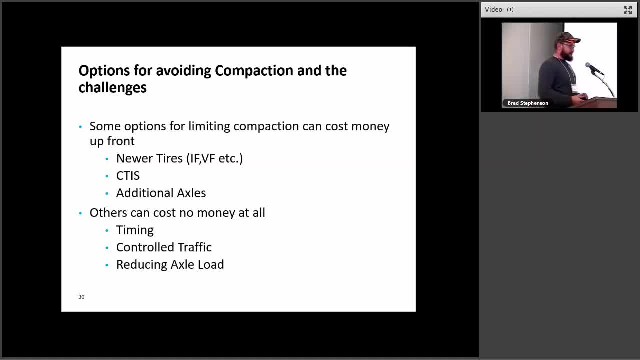 compaction, uh issues after the fact. so I had started the the year, gonna preach on timing as much as I could, and then it kept raining in April, and then it kept raining in May, and then it kept raining in June, and I'm gonna look like a fool if I tell you to just keep, just keep, waiting. it'll. get dry, you'll be able to do it. um so, yes, compaction probably happened this year. um, um, like I say, the top soil, the top six inches, in my opinion, it's going to take care of itself through the natural cycle of root growth and and- uh, if you're into, you know, some amount of tillage, or 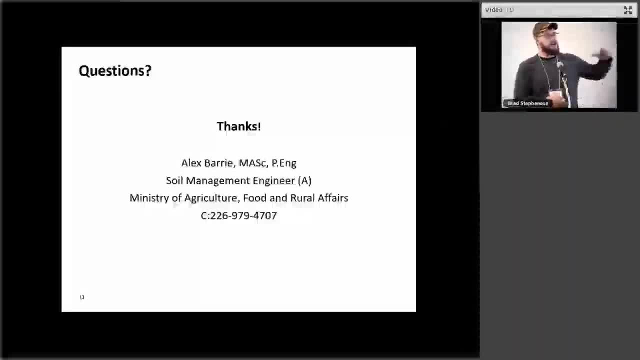 minimum tillage or no till, that top soil does rebound and we saw that and all that the year after. um there's a hit after compaction, but the following year it does rebound. um getting that middle depth layer uh fixed, uh, it's kind of kind of hard to do. 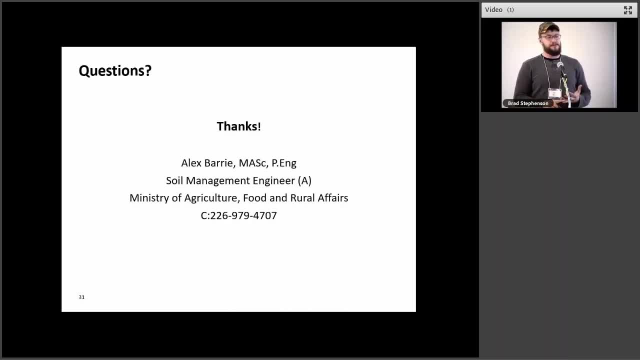 uh, aggressive rooting crops or cover crops so you can do the tillage radishes or the um the grasses or the the red clovers or whatever um. somebody asked me what's better: should I do like a tap root, real aggressive, deep, one root, or should I do some of that fibrous root system cover? 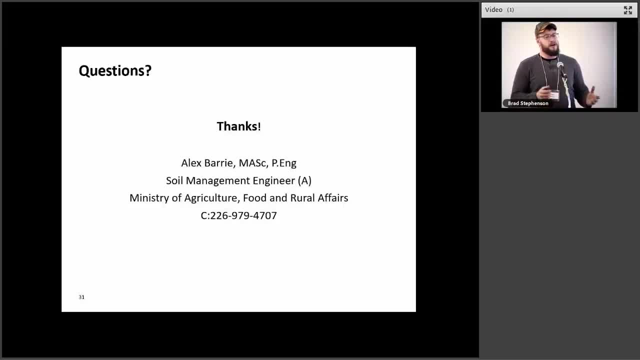 crop. I said: well, why not both? if you're repainting an old car, you're gonna strip all the paint, you're gonna put primer on it, then you're gonna paint it a different color. so each of those steps had a less. so if I was trying to remediate some deep compaction, I'd go in and I'd rip it up mechanically. till it, uh, fracture that compacted layer and then I would put in a deep rooting crop to get that stabilized kind of quickly and then I can start adding different cover crops and different rooting structures to try to knit that soil back together. because if I just came in and ripped it all up I 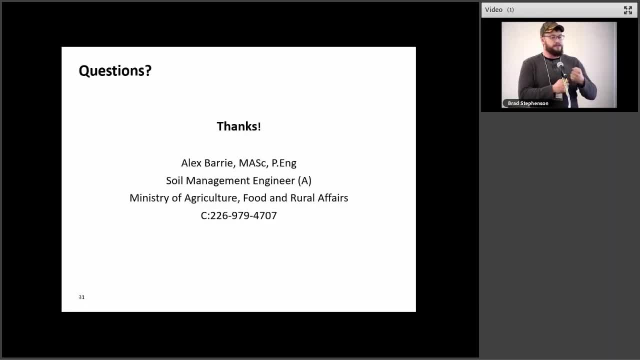 don't have any soil, I don't have any structure there, it's just like loose, loose aggregate or loose sand. it's going to just recompact. it's not going to have much strength after that at all. so you wouldn't just sandblast a car and leave it out. the fence bottom it'll rust. so the same kind of rules apply. 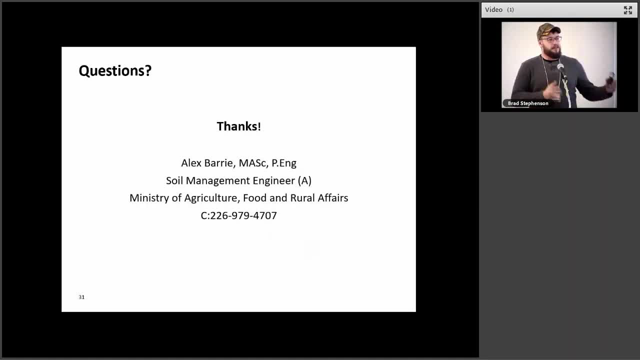 you can't just do really aggressive tillage and think that that solved your problem. you have to kind of provide some structure to the soil. so based on what I'm hearing you say, Alex is having perennial crops with deep tap roots and lots of fibrous root structure is a good thing. 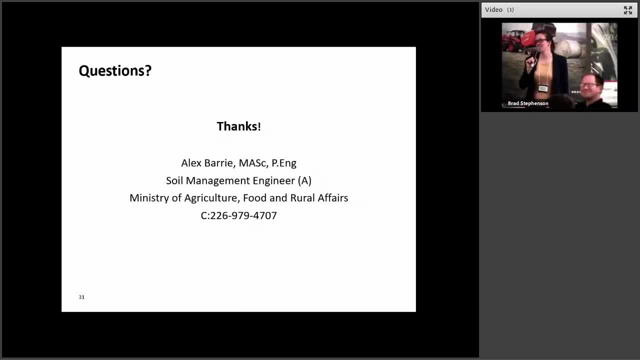 yes, okay, thanks. just we're a different audience than you usually give this talk to, so I wanted to like bring this back full circle- that we were growing crops that, given a chance you're growing, that are generally helpful and you're usually doing it on a timescale that is certainly helpful. 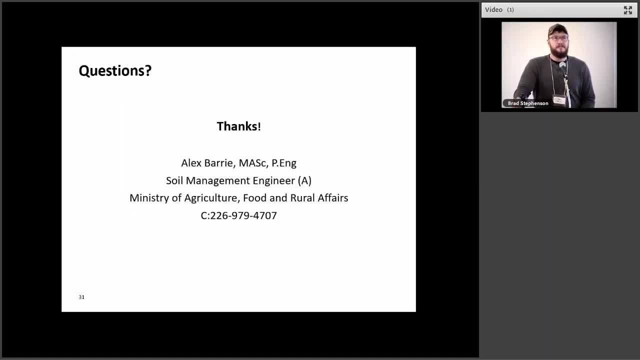 so in a straight soybeans, corn wheat rotation or, heaven forbid, a corn snow corn rotation, you're not going to take your soil and you're going to have to just sort of do a little bit of what you that land out of production and put hay in it for two years if you got nothing. 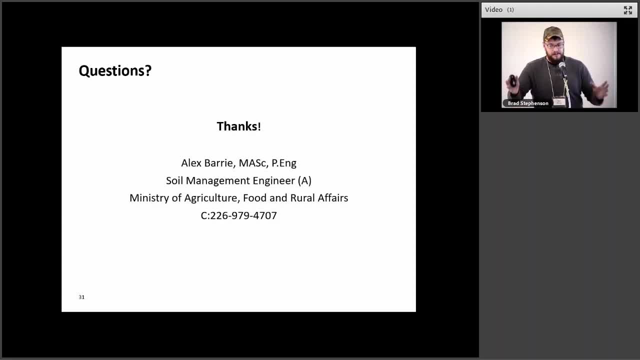 to feed the hay to. so in our end, and the case where you're growing forages for multiple years, you are giving that a chance to establish them some rooting depth and some some fiber fill in your, your concrete matrix. okay, thank you. a great presentation question for those of us in the forage business. I know you've. done lots of different trials of different machines which are our most compacting machines, and any suggestions on how to make them better. so the worst- probably not surprising, but it's not going to be very beneficial to you- is hay wagons. if you try to put 12 big square bales on 411 L tires at 60 or 70. 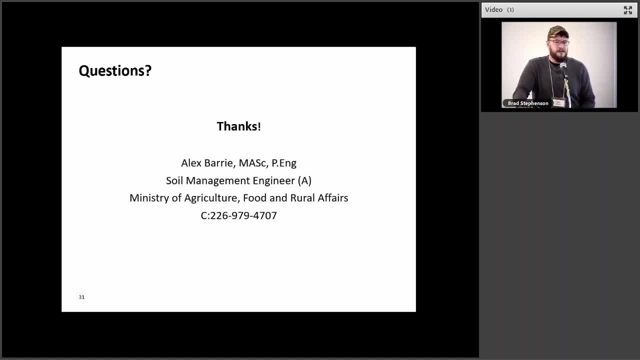 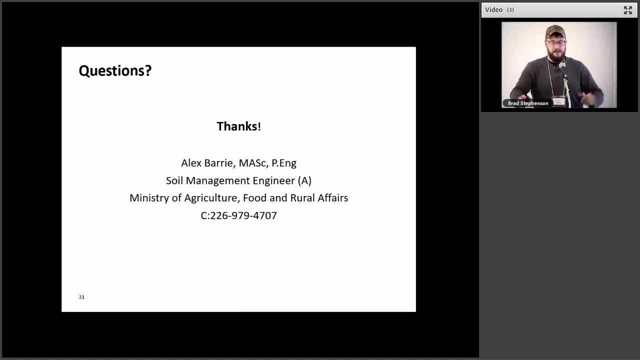 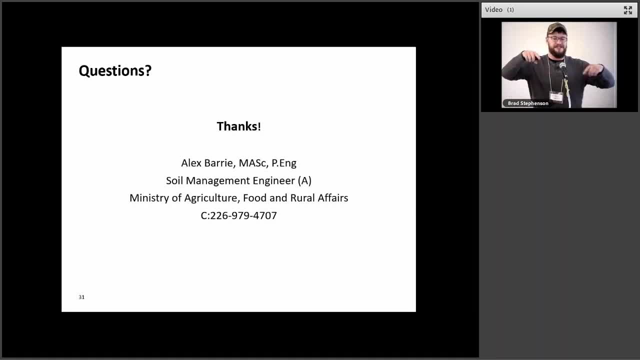 compaction you're going to do with all that. but the next year you're gonna see all those little wheel tracks through the field where you drove that hay wagon around through it. so the general rule- and this is true for all profiles, that soil profiles we've done wagons- think you're high pressure, 11 L tires, anything. 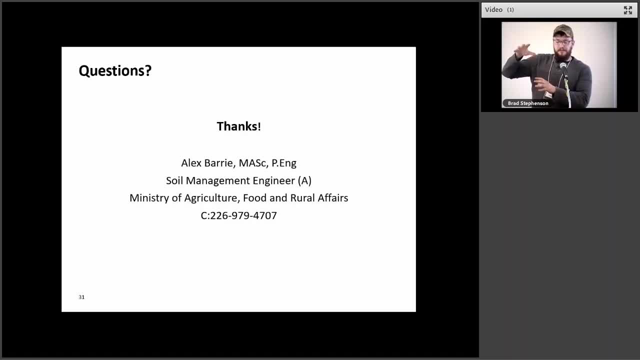 with those on it. you've got your high-value sprayers. you got you kind of your grain carts and your poorly set up manure spreaders are next. then you have your well set up tractors, sort of the lighter pieces of equipment like your pickup trucks kind. 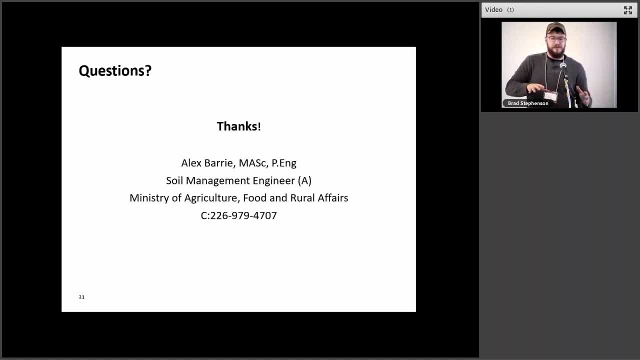 of down and a pickup truck in a well set up tractor is about equivalent as far as the top 12 inches go and then down from there to all the lighter stuff. so really if if you're looking at a piece of equipment and you see it's a nice little, 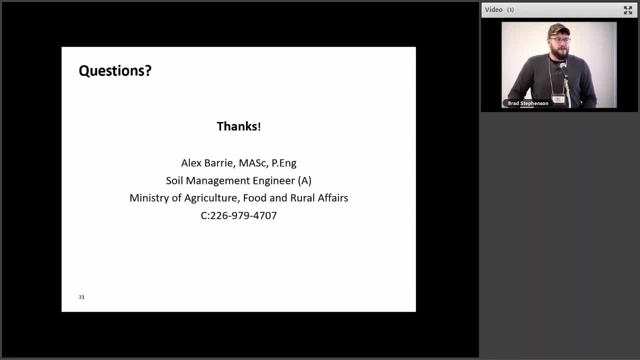 this is, this is kind of a priority. so the sugar co-op was making a bail mover and they wanted to. what are we doing right? what are we doing wrong? and I said: well, you've got a pretty decent tire on it, 18 psi, that's pretty good, you've got three axles. but to 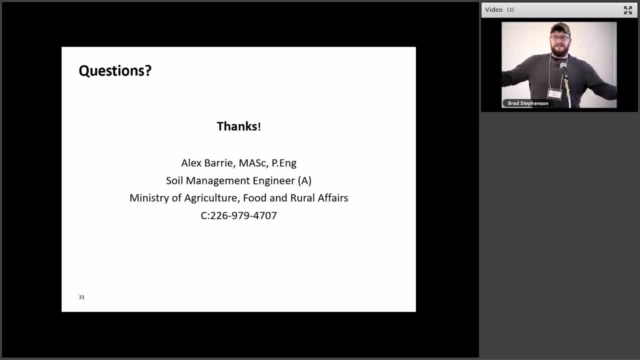 me this: looks like you can put six more bales on it, like with the axles you got. it looks like you don't have enough bales on it, so you put, you know, six more bales on it. well then, then you just hurt yourself because you've just increased the axle weight too much, so we got to get out of that that. 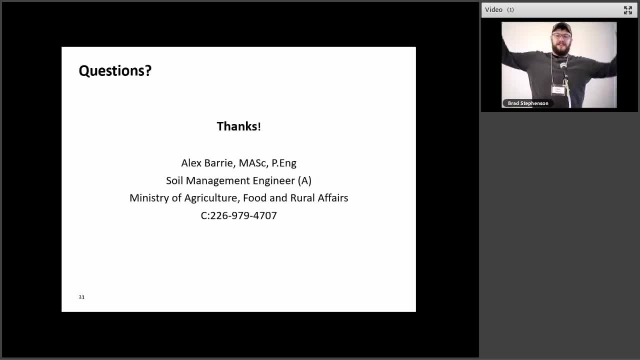 thinking where, oh, that looks like I could load that, you know, to the hill. but managing the axle weight is going to become as we move forward. you're gonna see a lot more tires under stuff. so that was a wild tangent. but hopefully that helps or doesn't. sure was one last question, if I may. 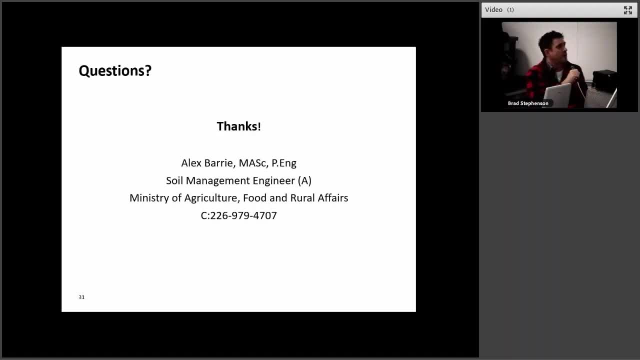 it's from our friends down in Ridgetown, and in one sentence or less, since it's already 302, how can one assess whether or not they've got a compaction problem in the first place? so one of my. this is not going to be one sentence. we're trying to set up a bit of a test and I'm trying to set 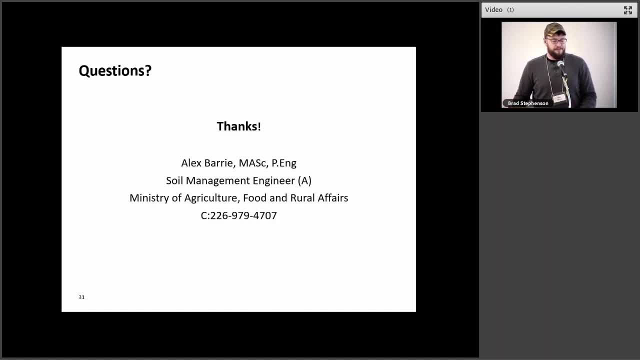 up a bit of a test that folks can do at home. we've got a lot of tests for a lot of other things. you know, throw the hoop out in your field and there's apps for measuring grass stands and whatever, but there's no real good test other than the Dickie John probe or the even just a tile probe. so go. 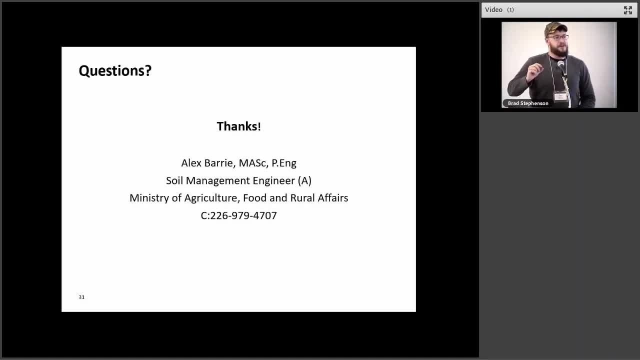 on the outside a little bit of a 5- 16th tip, to the end a little bigger diameter tip, and now you can use that to sort of compare your compacted areas to your not compacted areas. so go into your fence row and just sort of try to push that that tool into the ground and get a feel for what that feels.